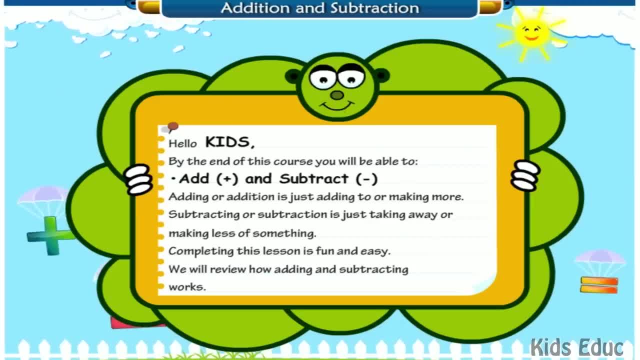 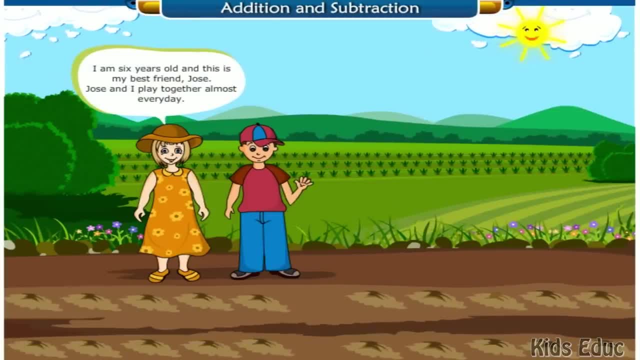 We will review how adding and subtracting works. Hello, My name is Annie, I am six years old and this is my best friend, Jose. Jose and I play together almost every day. We both like to grow a garden. Jose and I are going to plant a garden and we want you to help us. 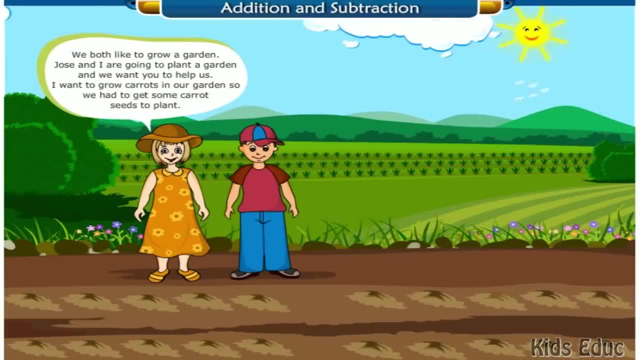 I want to grow carrots in our garden so we had to get some carrot seeds to plant. I have six carrot seeds. I have four carrot seeds. If I take my carrot seeds and add them to Jose's carrot seeds, how many carrot seeds will I get? 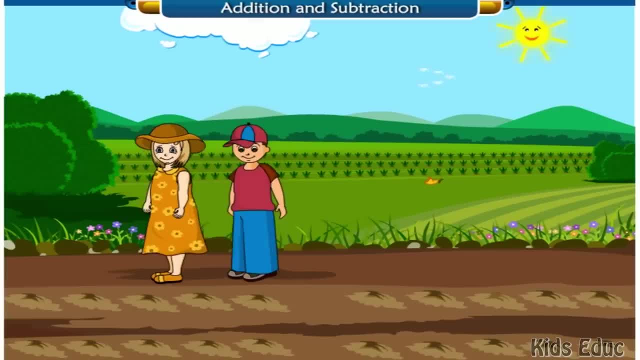 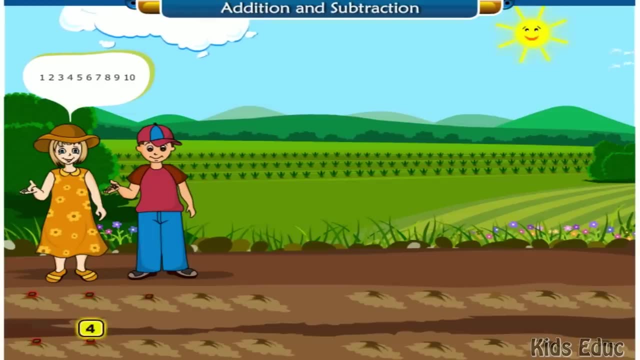 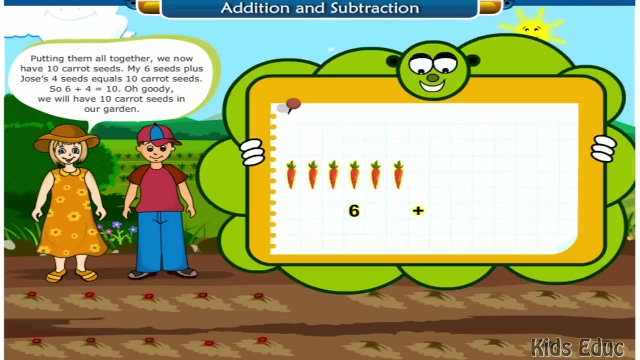 How many carrot seeds? How many carrot seeds do we have? One, two, three, four, five, six, seven, eight, nine, ten. Putting them all together, we now have ten carrot seeds. My six seeds plus Jose's four seeds equals ten carrot seeds. 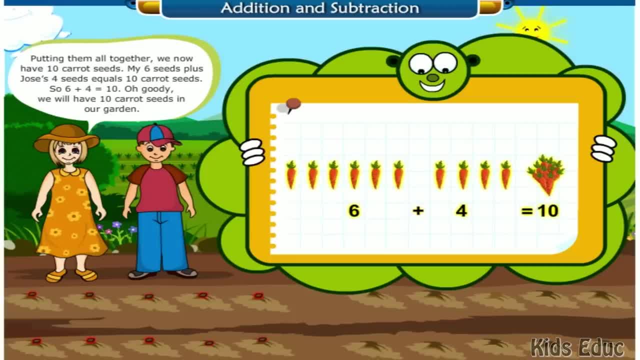 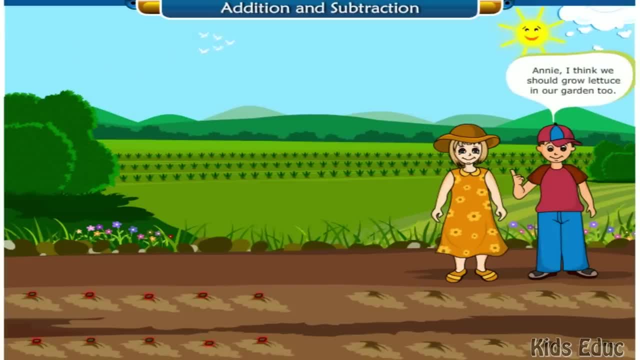 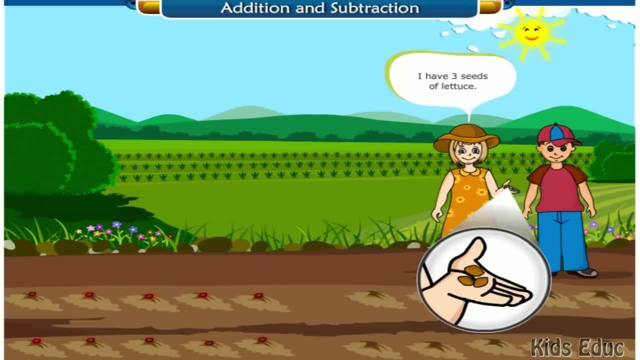 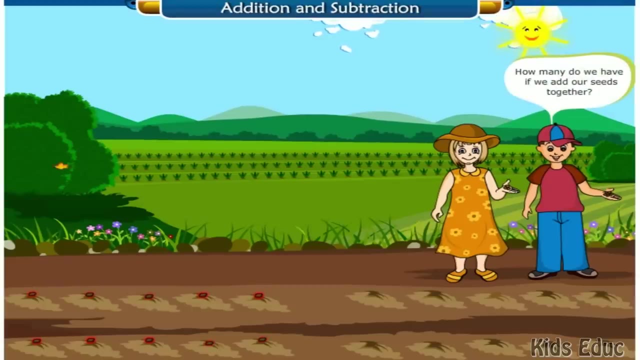 Annie, I think we should grow lettuce in our garden too. That sounds like a great idea. I have three seeds of lettuce. I have seven lettuce seeds. How many do we have if we add our seeds together? One, two, three, four, five, six, seven, eight, nine, ten? 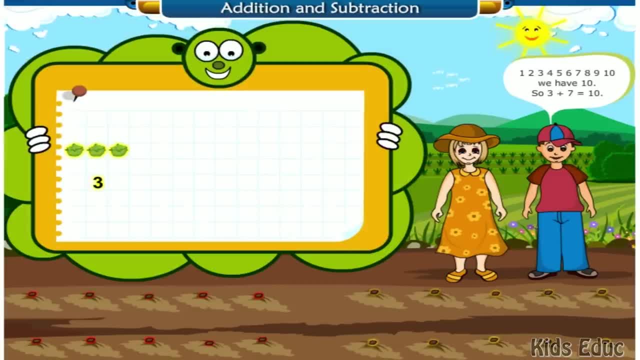 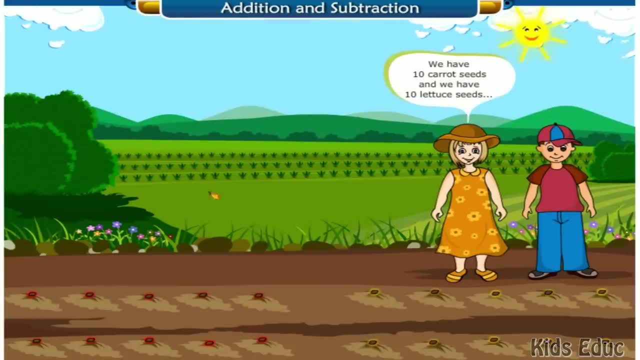 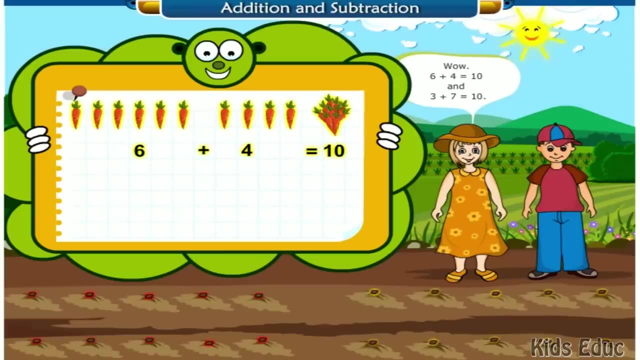 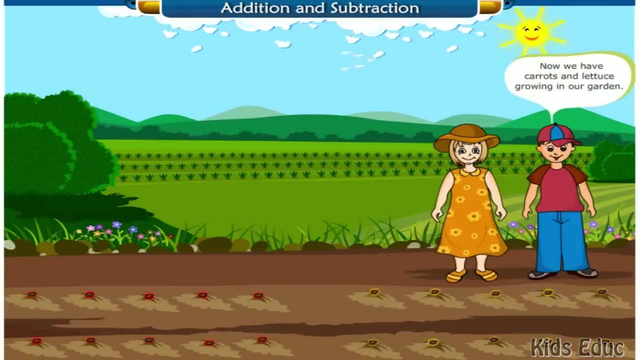 We have ten. So three plus seven equals ten. We have ten carrot seeds and we have ten lettuce seeds. Wow, Wow, 6 plus 4 equals 10, and 3 plus 7 equals 10.. Now we have carrots and lettuce growing in our garden. 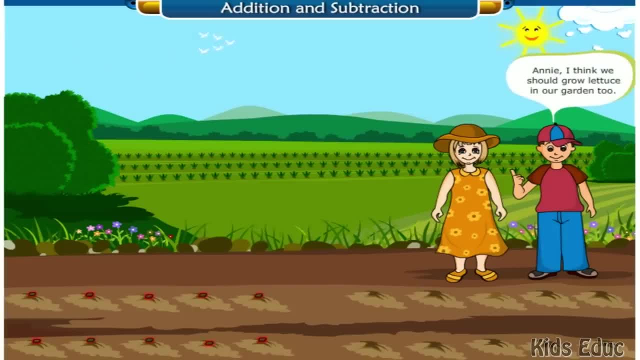 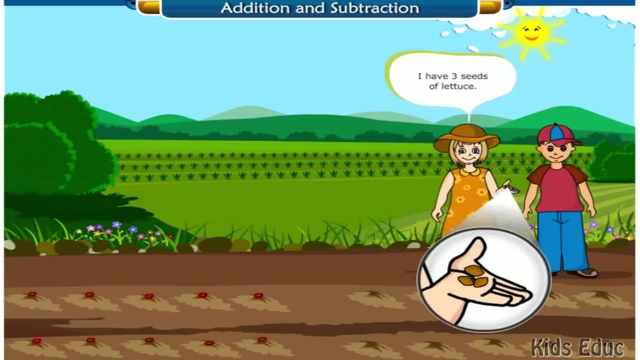 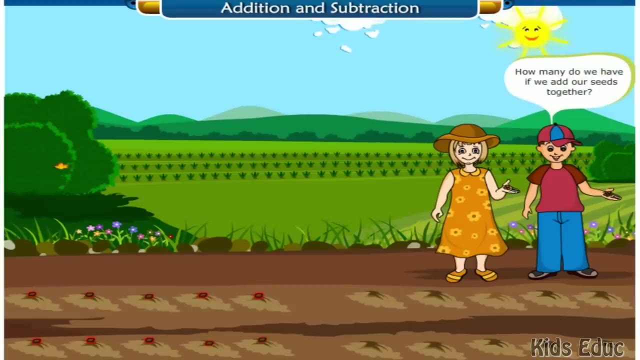 Annie, I think we should grow lettuce in our garden too. That sounds like a great idea. I have three seeds of lettuce. I have seven lettuce seeds. How many do we have if we add our seeds together? One, Two, Three? 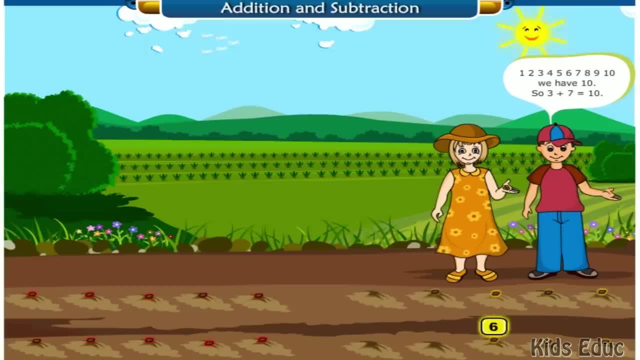 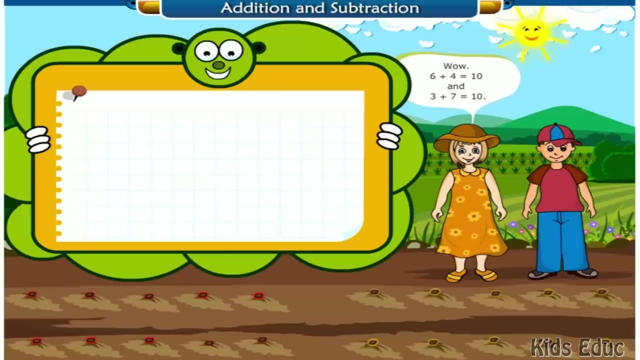 Four, Five, Six, Seven, Eight, Nine, Ten. We have ten. So three Plus seven equals ten. We have ten carrot seeds and we have ten lettuce seeds. Wow, Six, Six plus four equals ten, and three plus seven equals ten. 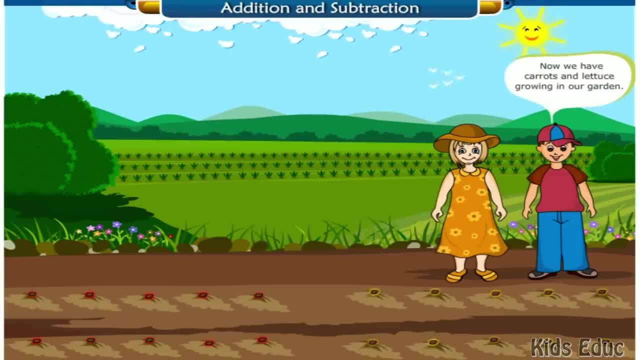 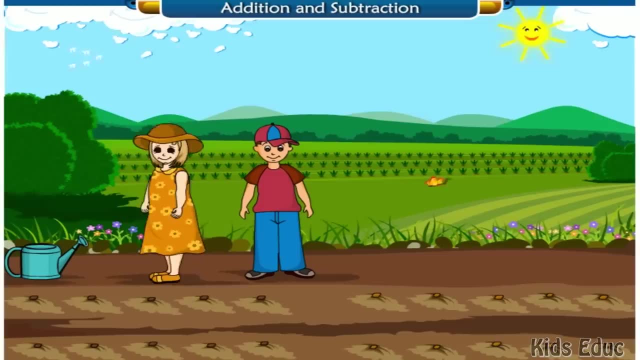 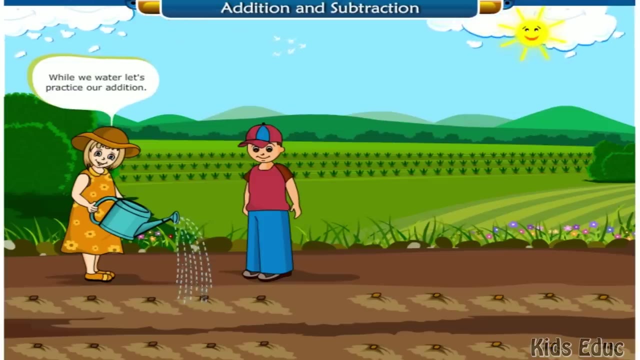 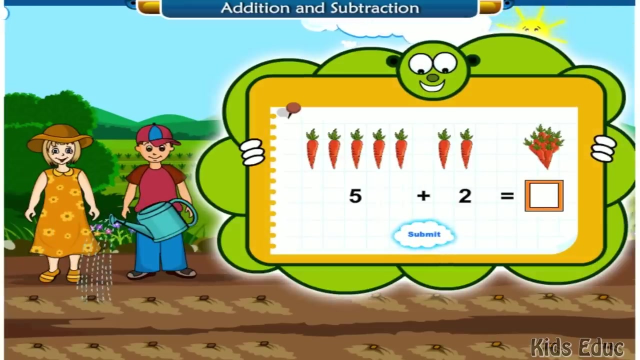 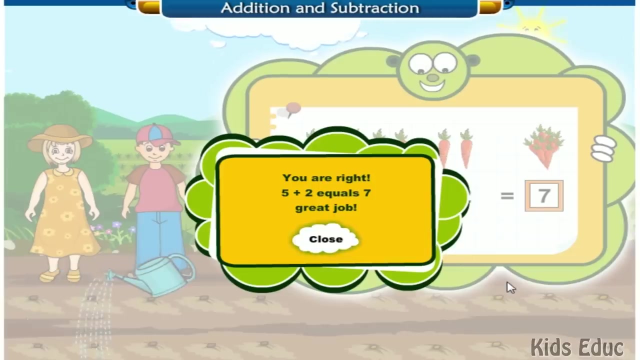 Now we have carrots and lettuce growing in our garden. Now we need to water the seeds, so they will grow While we water. let's practice our addition: Five carrots plus two carrots equals. You are right, Five plus two equals seven. Great job. 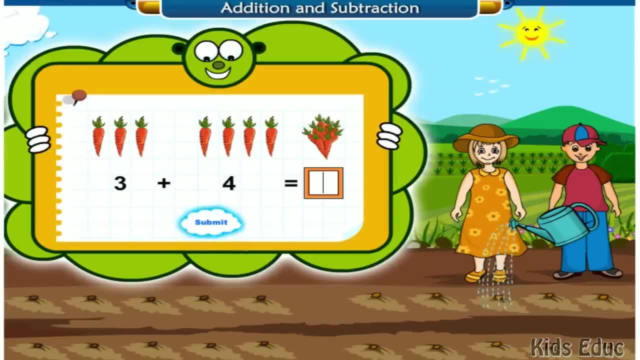 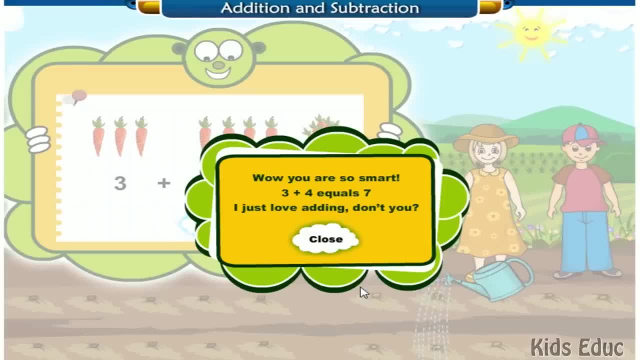 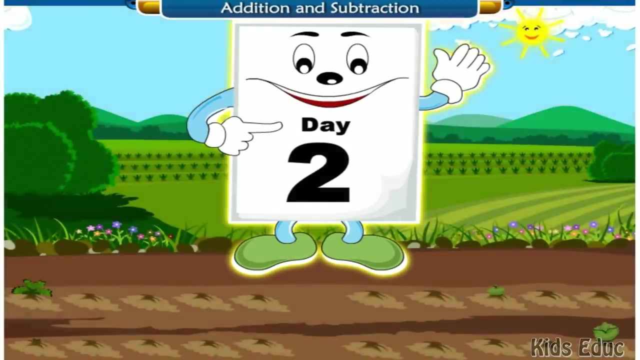 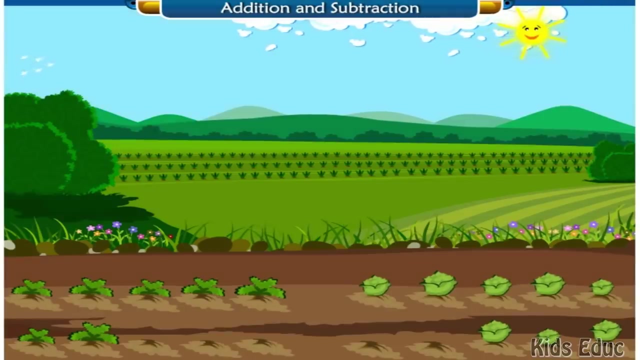 Three carrots plus four carrots equals- Wow, You are so smart. Three plus four equals seven. I just love adding, don't you? Six plus four equals ten, and three plus seven equals ten. Jose, Jose, look, We have some carrot plants. 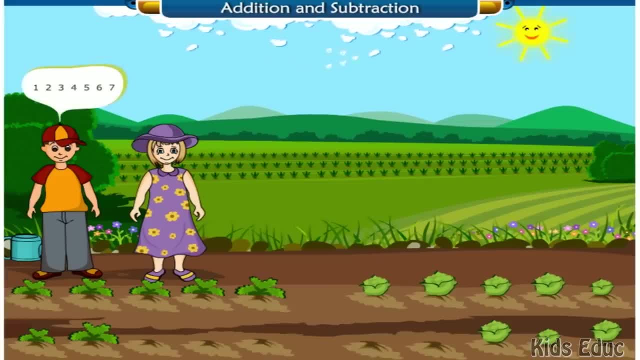 Let's count how many plants we have: One, two, three, four, five, six, seven. We have seven carrot plants, Jose. how many seeds do you have? Six plus two equals ten. Great job did we plant? we planted 10 carrot seeds. so if we planted 10 carrot seeds and we 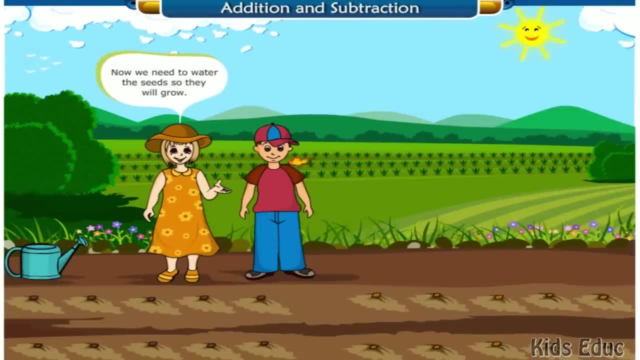 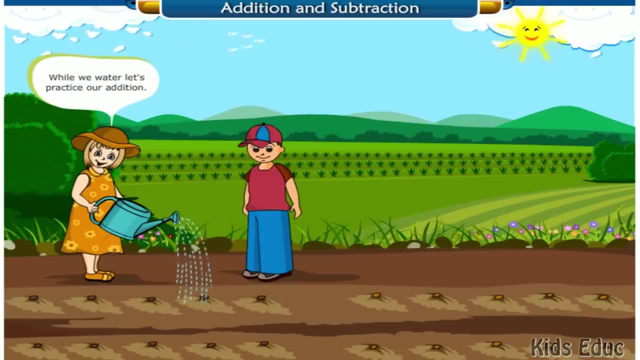 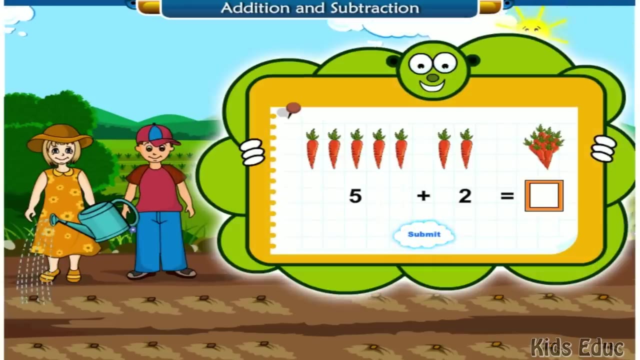 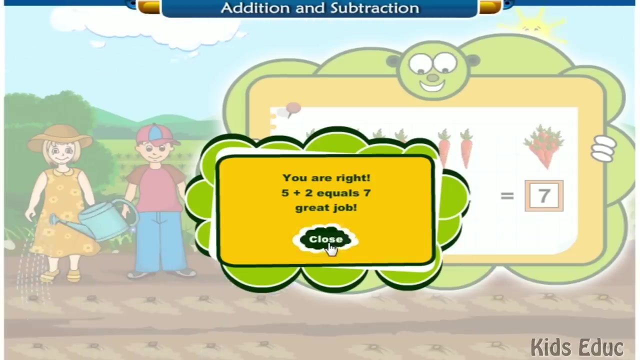 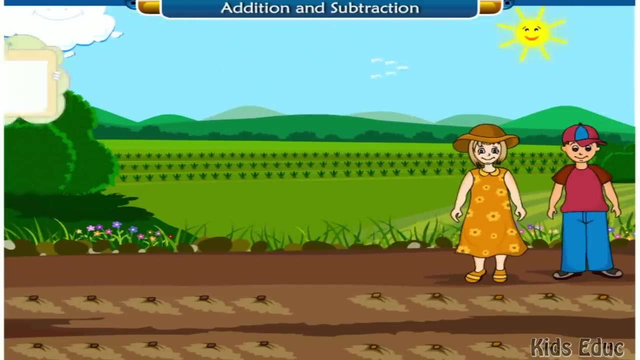 Now we need to water the seeds, so they will grow While we water. let's practice our addition: 5 carrots plus 2 carrots equals. You are right, 5 plus 2 equals 7.. Great job. 3 carrots plus 4 carrots equals. 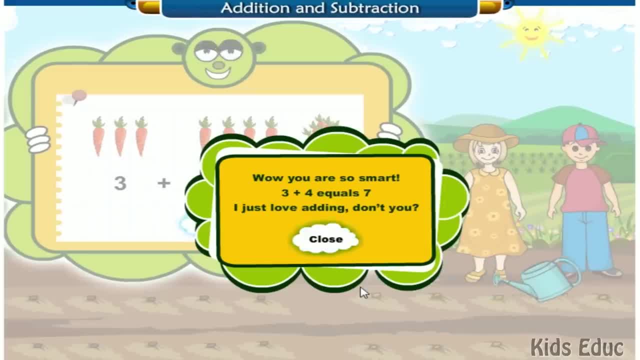 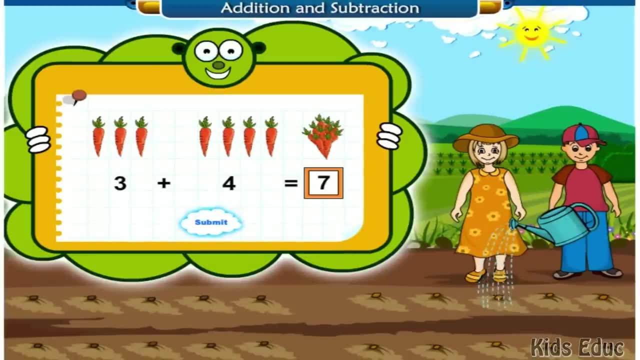 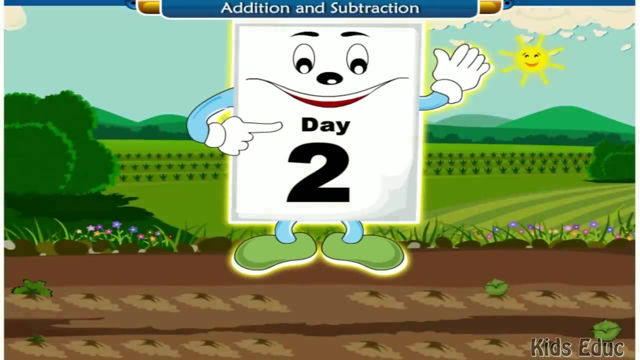 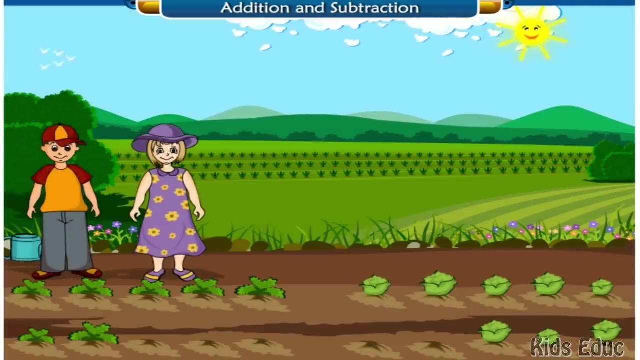 Wow, You are so smart. 3 plus 4 equals 7.. I just love adding, don't you, Jose? Jose, look, We have some carrot plants. Let's count how many plants we have: 1,, 2,, 3,, 4,, 5,, 6,, 7.. 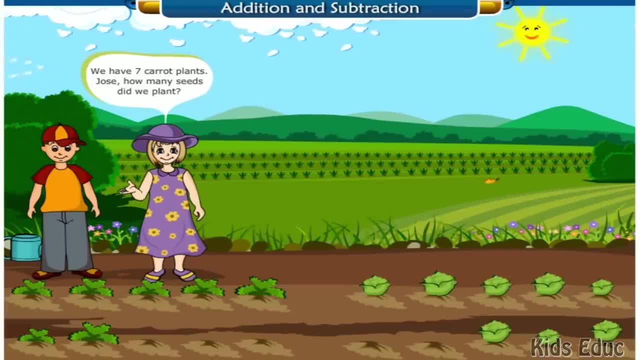 We have 7 carrot plants, Jose. how many seeds did we plant? We planted 10.. We planted 10 carrot seeds. So if we planted 10 carrot seeds and we only have 7 carrot plants, how many more carrot plants will grow? 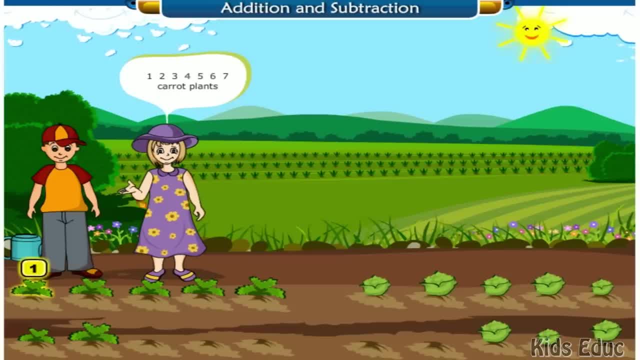 Let's see: 1,, 2,, 3,, 4,, 5,, 6,, 7 carrot plants, 8, 9,, 10 seedlings And 8 seedlings. contradiction: 7 carrot plants plus 3 carrot seeds. add 3 micron seedlings. add. 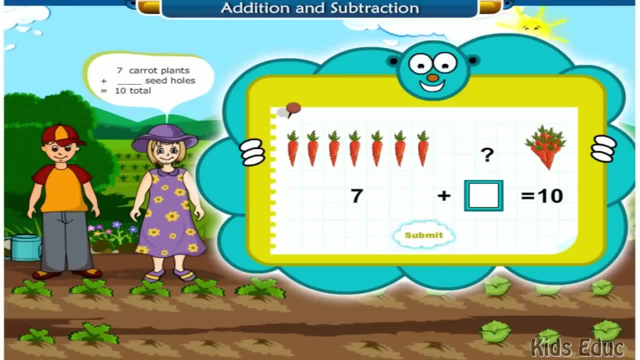 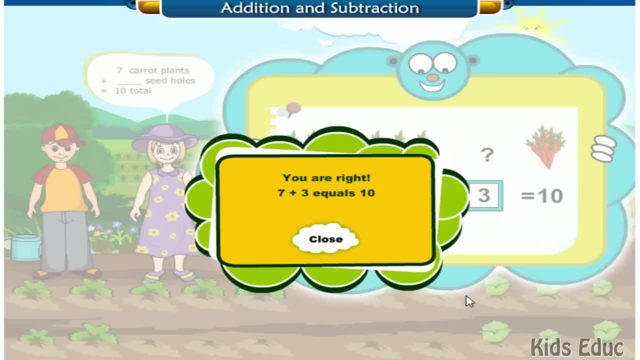 We'll multiply seed. So 7 carrot plants plus 7 carrot seeds equals 10 total. No, we're multiplying the photos: 7 carrot plants plus seed holes, Not left right. Let's start out counting more seedlings. 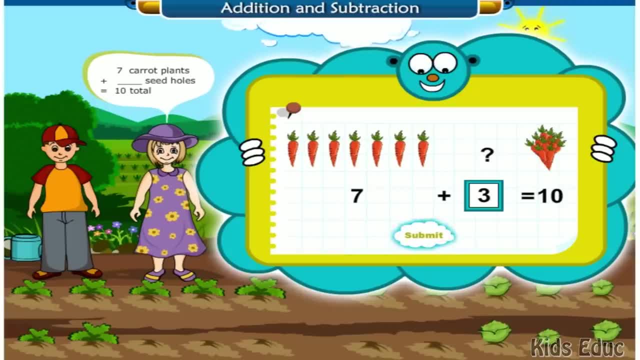 1,, 2,, 3,, 4, 5.. The cars we bed. we don't need molecules, we can put them inside the container. 2,, 3,, 4,, 5,, 6, 7 carrot seeds for their weight. 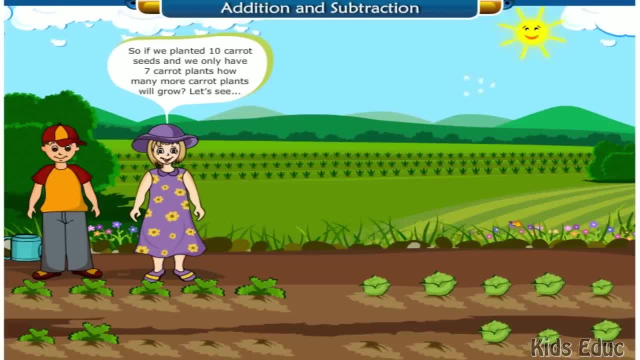 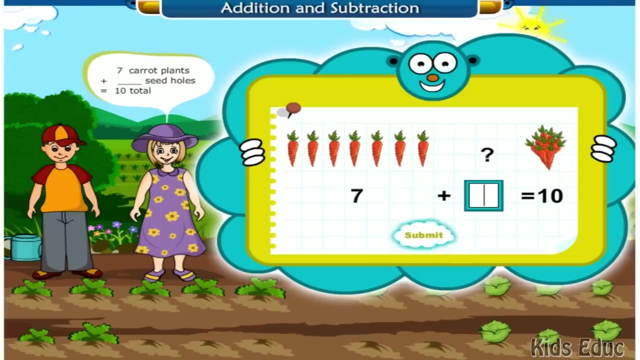 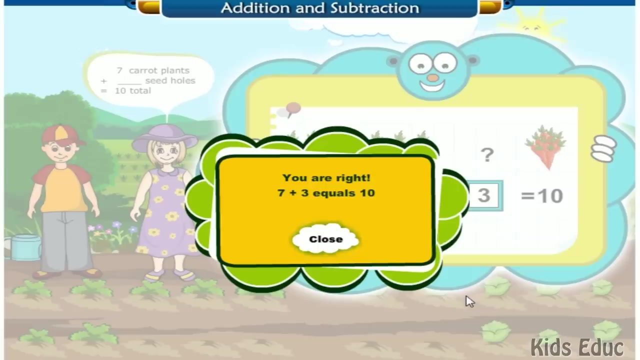 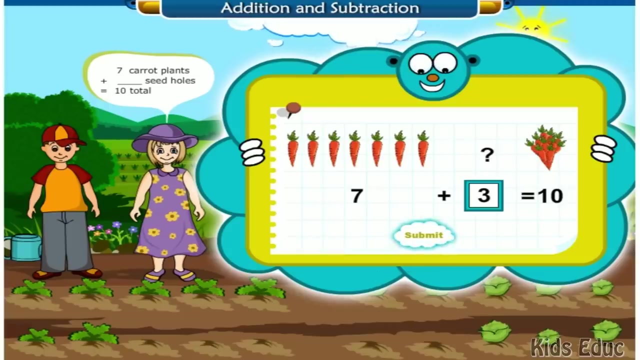 only have seven carrot plants, how many more carrot plants will grow? let's see: 1, 2, 3, 4, 5, 6, 7 carrot plants: 8, 9, 10 seed holes: 7 carrot plants plus seed holes equals 10 total. you are right, 7 plus 3 equals 10. 7 carrot plants plus 3 seed holes: equals. 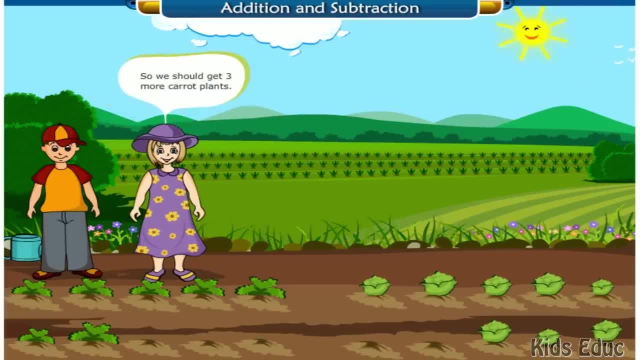 10 total. so we should get three more carrot plants. let's count our lettuce plants: 1, 2, 3, 4, 5, 6, 7 carrot plants plus 3 seed holes equals 10 total. so we should get 3 more carrot plants. let's count our lettuce plants: 1. 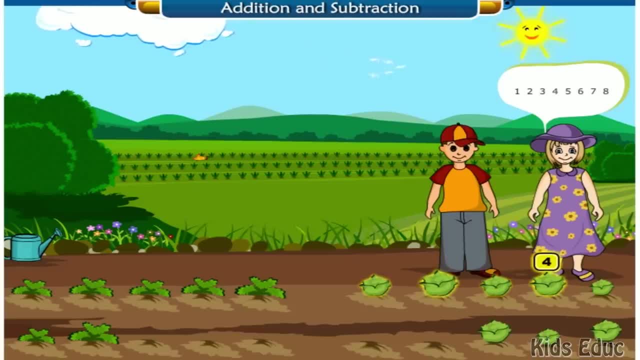 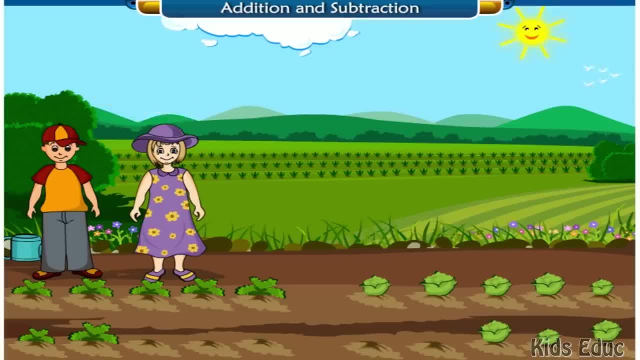 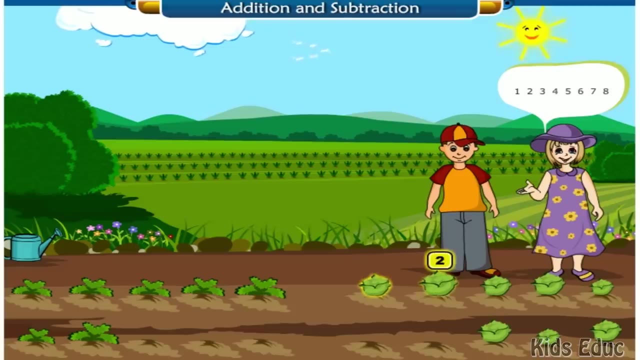 7 carrot plants plus 3 carrot seeds, 7 plus seed holes, make our pots 7 carrots plants plus 10 total, ten total. so we should get three more carrot plants. let's count our lettuce plants: one, two, three, four, five, six, seven, eight. we have eight lettuce plants, Jose. 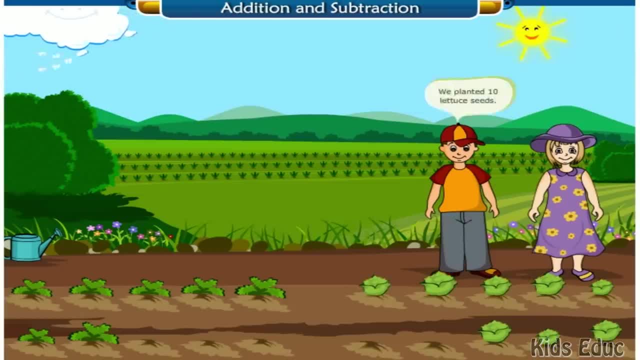 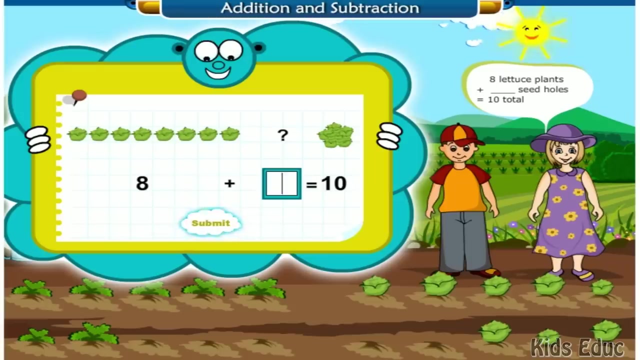 how many seeds did we plant? we planted ten lettuce seeds. so if we planted ten lettuce seeds and we have only eight lettuce plants, how many more lettuce plants will still grow? let's see one, two, three, four, five, six, seven, eight lettuce plants, nine, ten seed holes, eight lettuce plants plus seed holes, equals ten total. 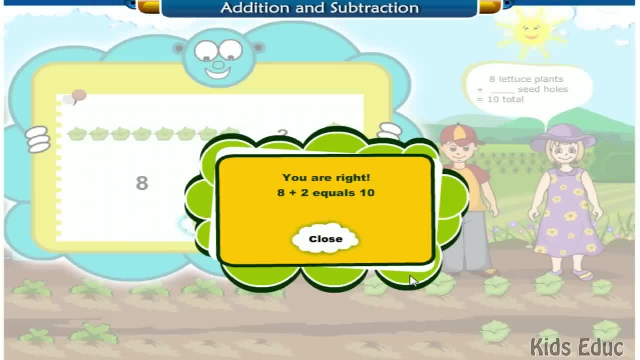 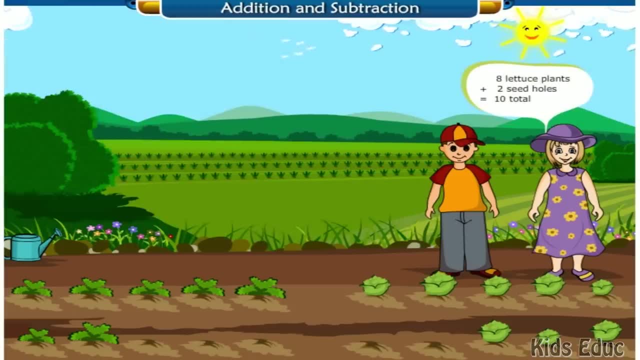 you are right. eight plus two equals ten. eight lettuce plants Plus two seed holes equals ten total. So we should get two more lettuce plants. Great job, Jose, and I really like adding and subtracting. It is so much fun. We better water our garden again. 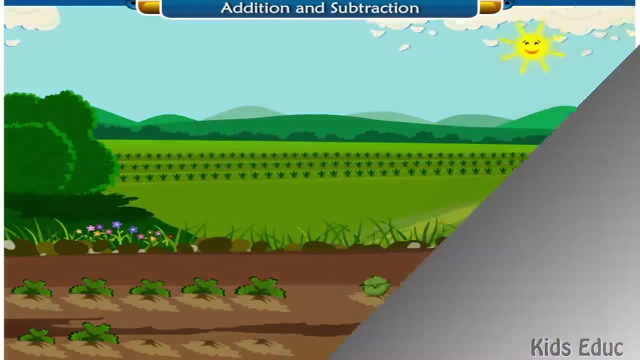 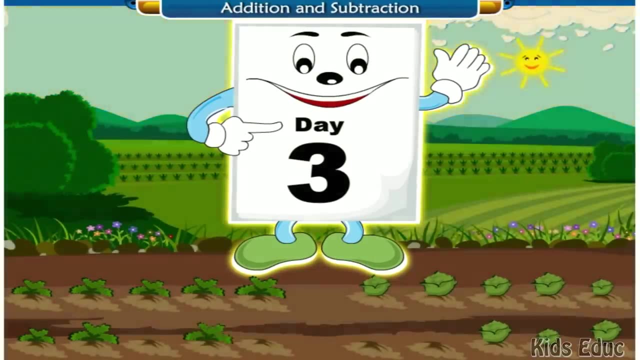 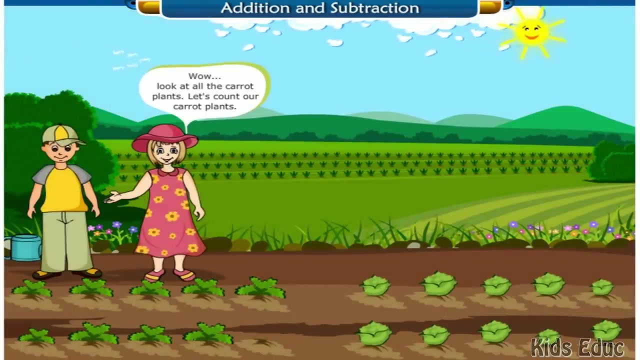 Our plants get very thirsty. Wow, Look at all the carrot plants. Let's count our carrot plants: One, two, three, four, five, six, seven, eight, nine, ten, Nine. We have nine carrot plants now. 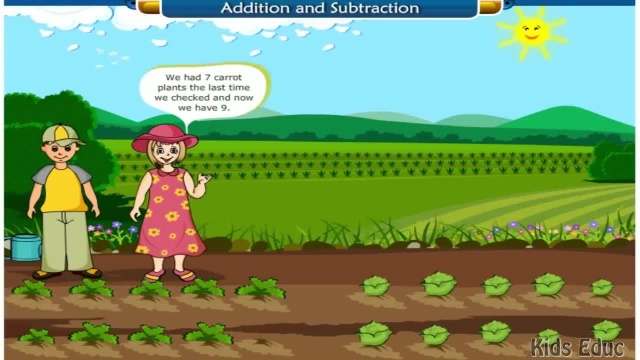 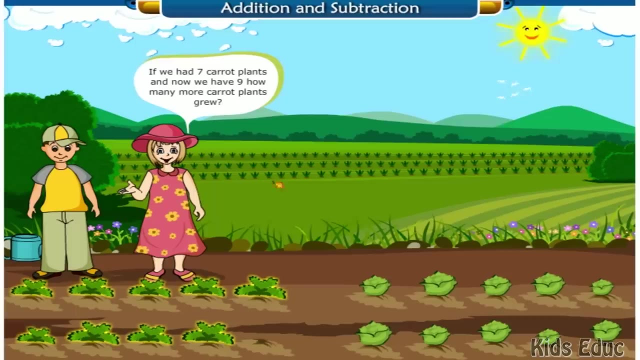 We had seven carrot plants the last time we checked, and now we have nine. Jose, how many more carrot plants grew since we checked our garden? Let's see If we had seven carrot plants and now we have nine, how many more carrot plants grew? 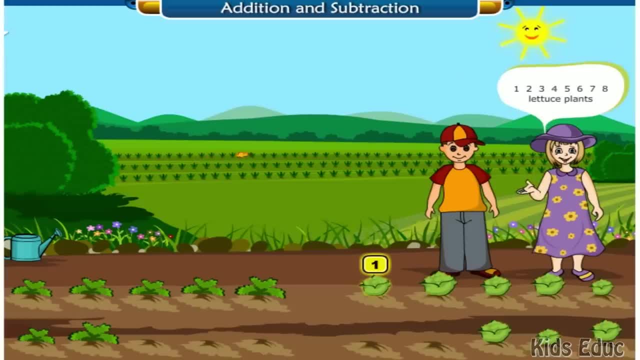 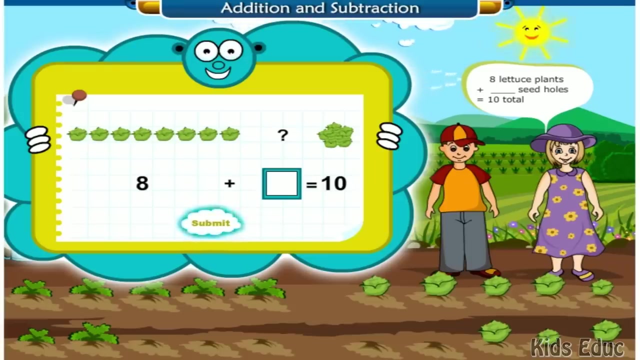 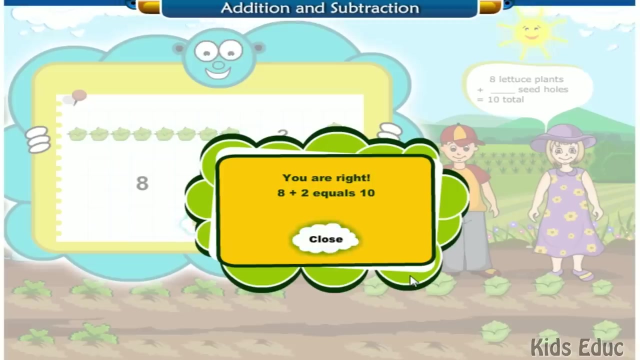 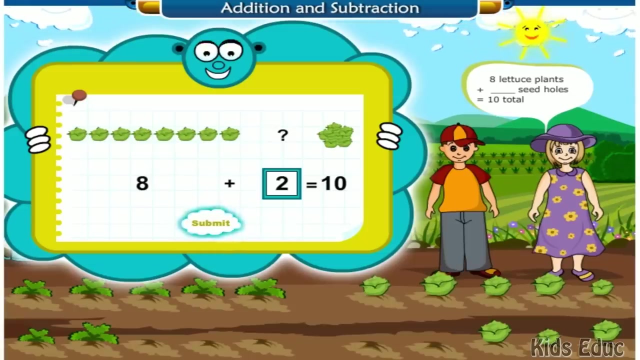 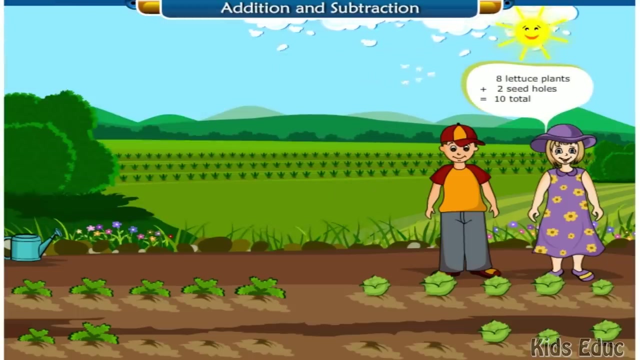 let's see one, two, three, four, five, six, seven, eight lettuce plants, nine ten seed holes. eight lettuce plants plus seed holes equals ten total. you are right, eight plus two equals ten. eight lettuce plants plus two seed holes equals ten total. so we should get two more lettuce plants. great job, Jose, and I really like adding and subtracting. it is. 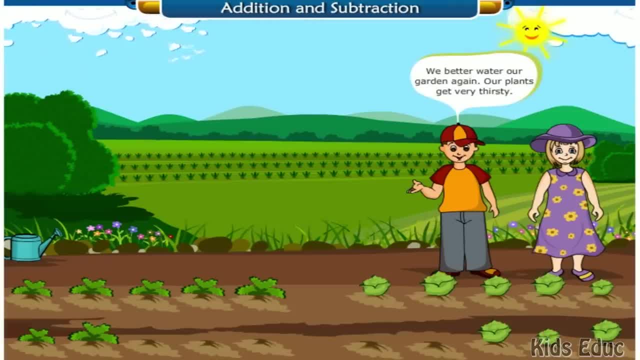 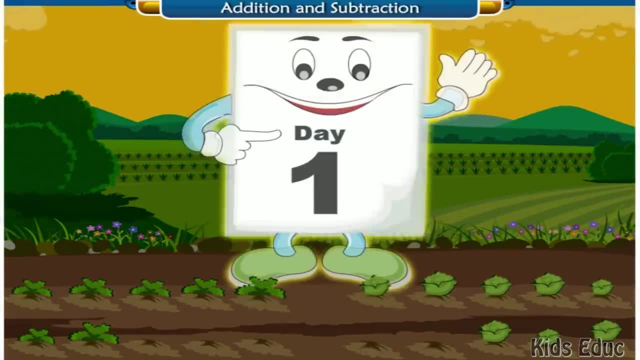 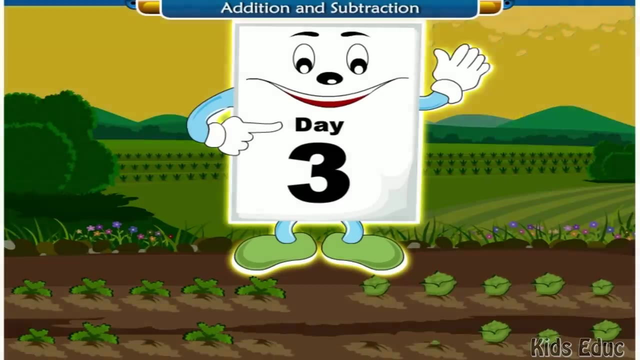 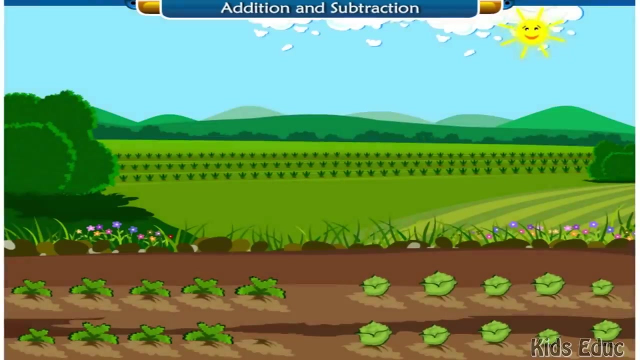 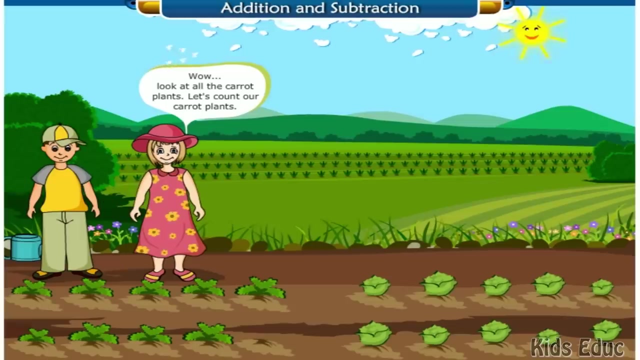 so much fun, we'd better water our garden again. our plants get very thirsty. Wow, look at all the carrot plants. let's count our carrot plants: one, two, three, four, five, six, seven, eight, nine. we have nine carrot plants now. we had seven carrot plants the last time we 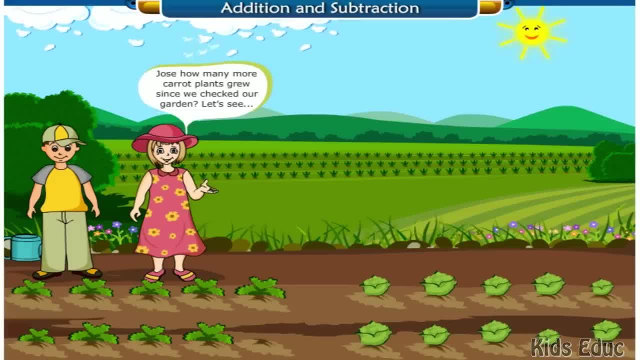 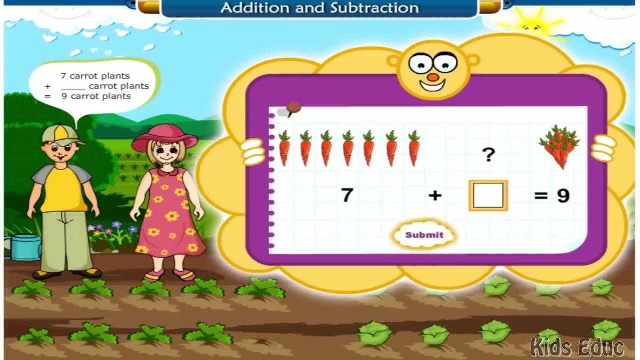 checked and now we have nine. Jose, how many more carrot plants grew since we checked our garden? let's see If we had 7 carrot plants and now we have 9,. how many more carrot plants grew? 7 carrot plants plus carrot plants equals 9 carrot plants. 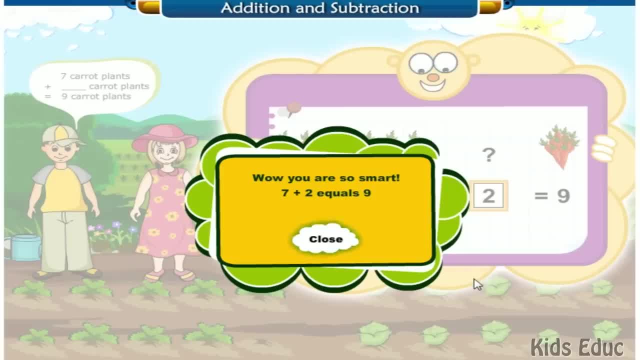 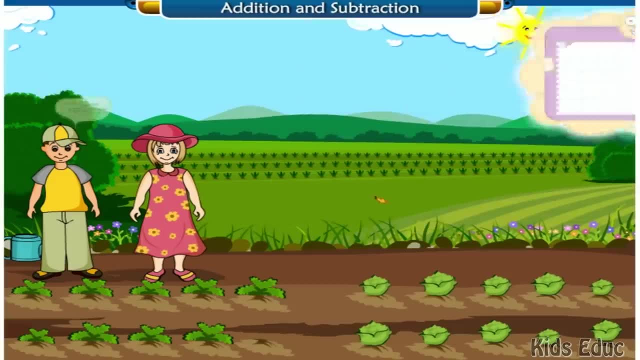 Wow, you are so smart. 7 plus 2 equals 9.. 7 carrot plants plus 2 carrot plants equals 9 carrot plants. 2 more carrot plants grew. The answer is 2. Great job. Now how many more carrot seeds still need to grow? 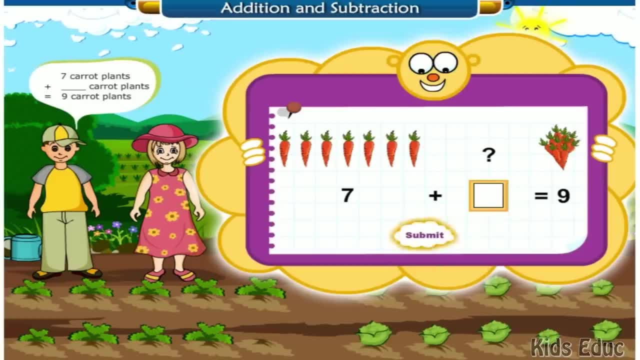 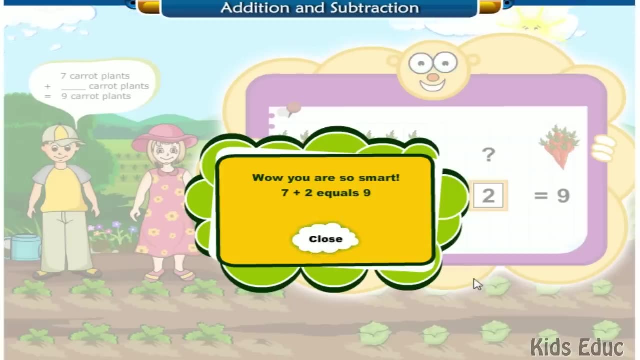 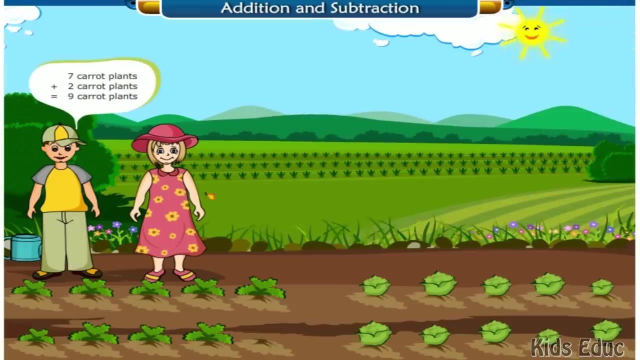 Seven carrot plants plus carrot plants. Nine carrot plants equals nine carrot plants. Wow, You are so smart. Seven plus two equals nine. Seven carrot plants plus two carrot plants equals nine carrot plants. Two more carrot plants grew. The answer is two. 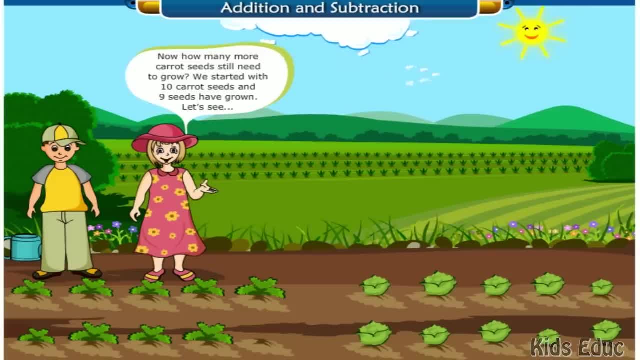 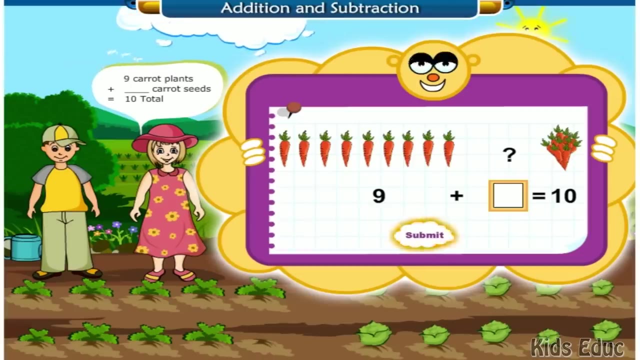 Great job. Now, how many more carrot seeds still need to grow? We started with ten carrot seeds and nine seeds have grown. Let's see: Nine carrot plants plus carrot seeds equals ten total. You are right, Nine plus one equals ten. 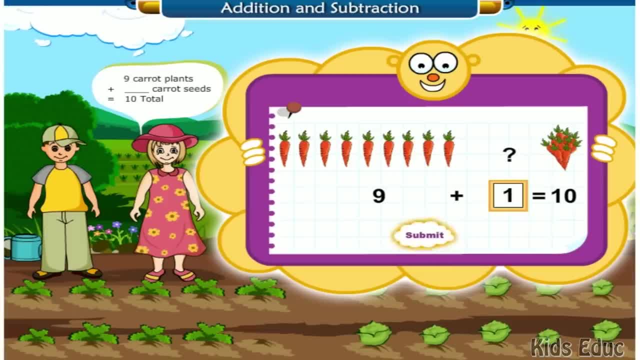 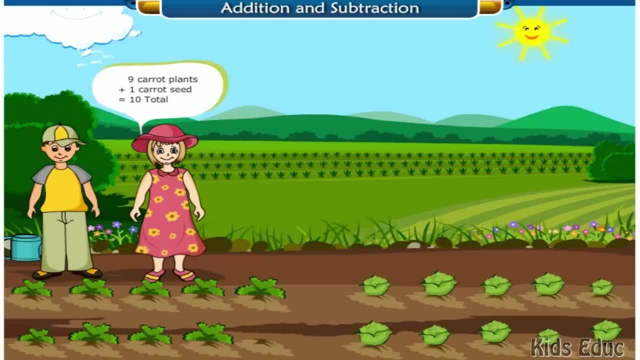 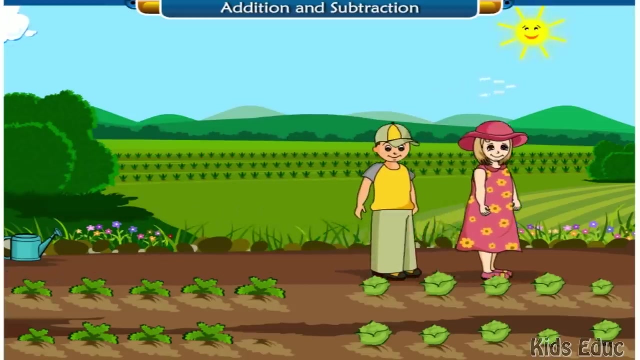 Ten Nine carrot plants plus one carrot seed equals ten total. We have just one more carrot seed that still needs to grow. Yay, Let's count how many lettuce plants have grown. One. How many lettuce plants did we have the last time we checked? 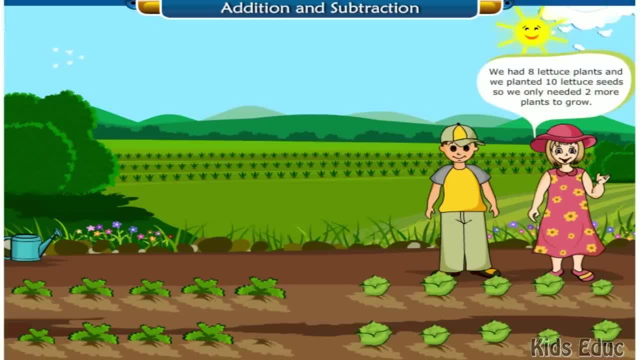 We had eight lettuce plants and we planted ten lettuce seeds, so we only needed two more plants to grow. Wow, Jose, We now have one, two, three, four, five, six, seven, eight, nine, ten lettuce plants. 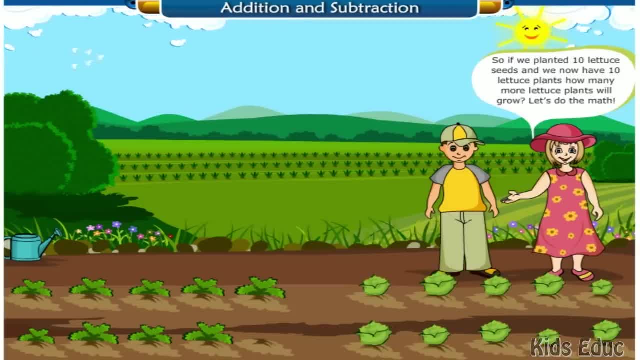 Ten lettuce plants. So if we planted ten lettuce seeds, we would have six, seven, eight, nine, ten lettuce seeds. If we planted 10 lettuce seeds and we now have 10 lettuce plants, how many more lettuce plants will grow? 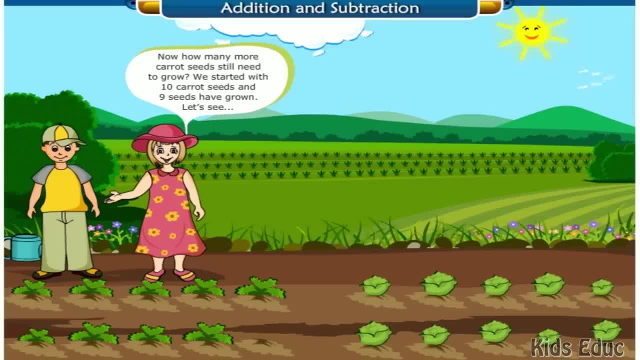 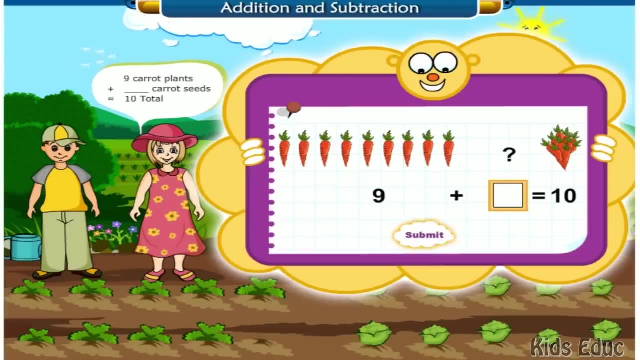 We started with 10 carrot seeds and 9 seeds have grown. Let's see: 9 carrot plants plus 2 carrot plants equals 9 carrot plants. 9 plus carrot seeds equals 10 total. You are right, 9 plus 1 equals 10.. 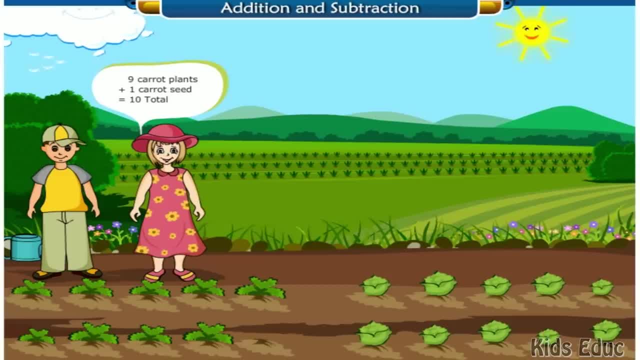 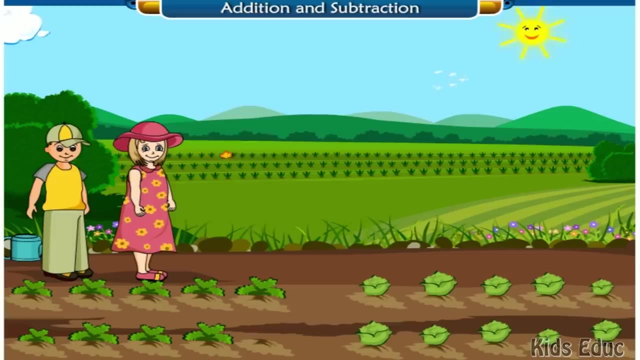 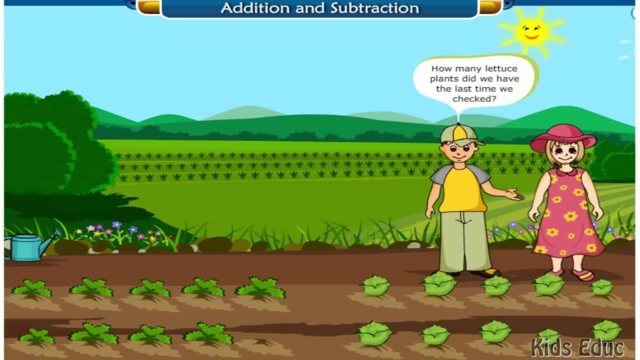 9 carrot plants plus 1 carrot seed equals 10 total. We have just 1 more carrot seed that still needs to grow. Yay, Let's count how many lettuce plants have grown. How many lettuce plants did we have the last time we checked? 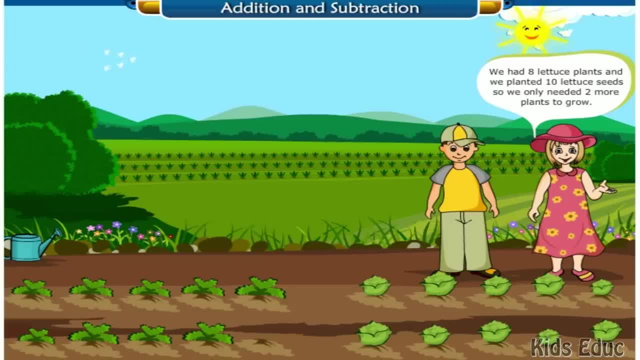 We had 8 lettuce plants and we planted 10 lettuce seeds, So we only needed 2 more plants to grow. Wow, Jose, We now have 1,, 2,, 3,, 4,, 5,, 6,, 7,, 8,, 9, 10 lettuce plants. 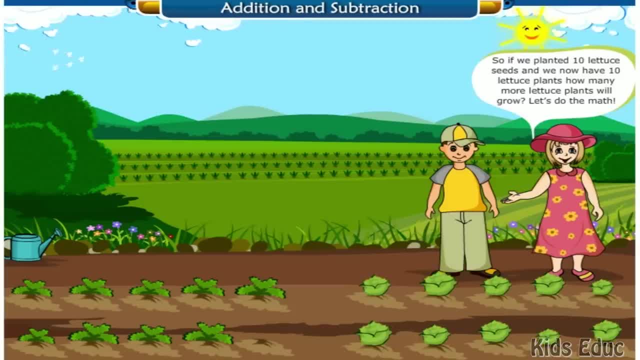 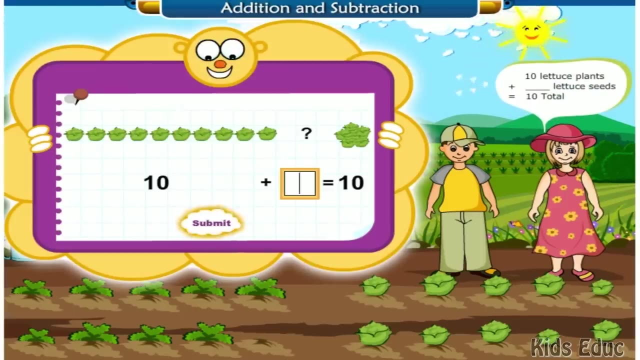 10 lettuce plants. So if we planted 10 lettuce seeds and we now have 10 lettuce plants, how many more lettuce plants will grow? Let's do the math: 10 lettuce plants, 10 lettuce plants plus lettuce seeds, equals 10 total. 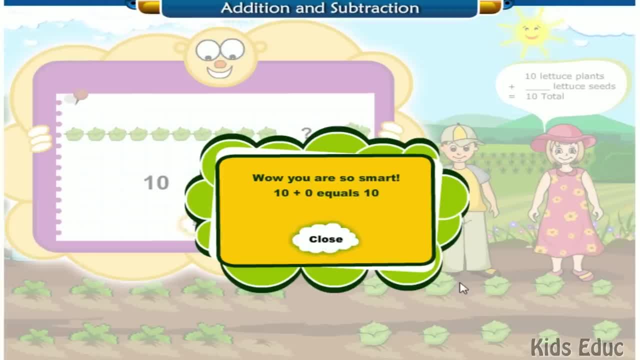 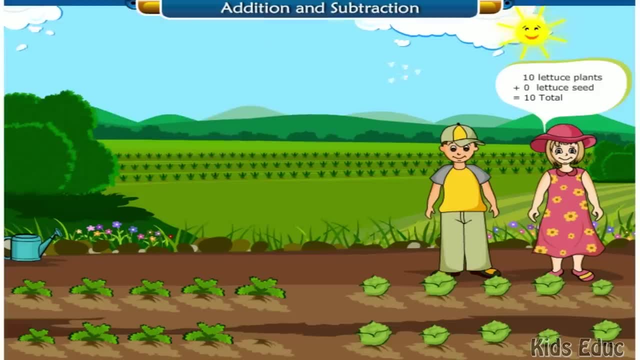 Wow, You are so smart. 10 plus 0 equals 10.. 10 lettuce plants plus 0 lettuce seeds equals 10 total. You are right. We have no more lettuce seeds to grow. You are so good at math. Let's water our garden, so all the seeds will grow big and strong. 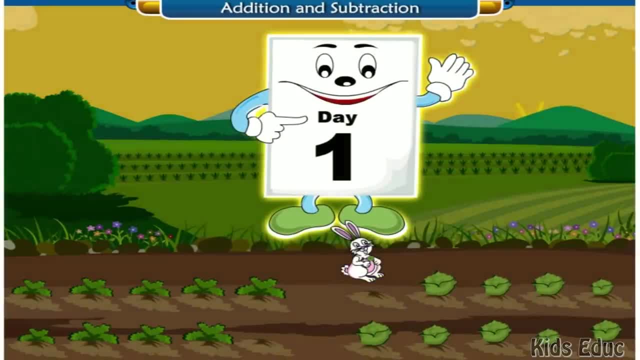 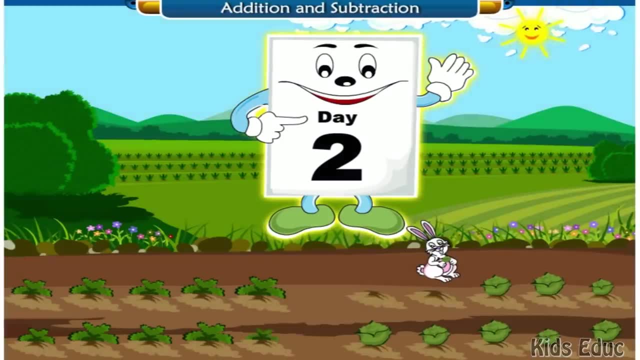 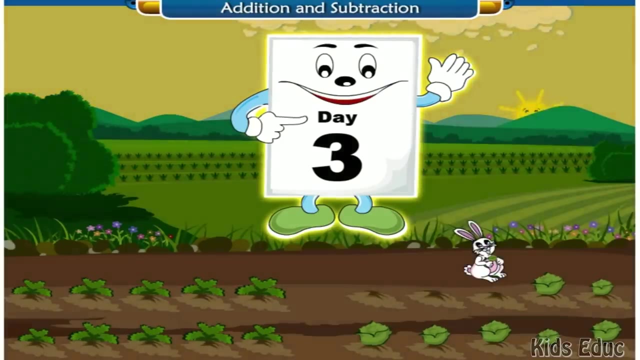 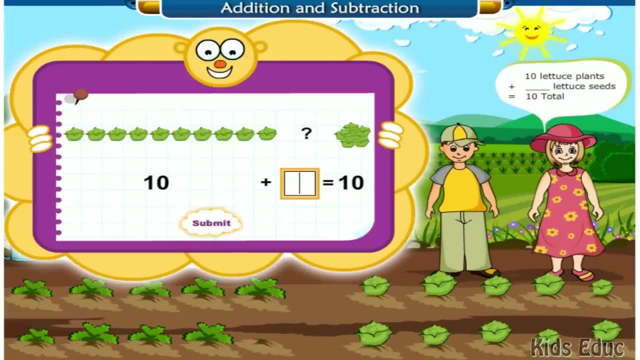 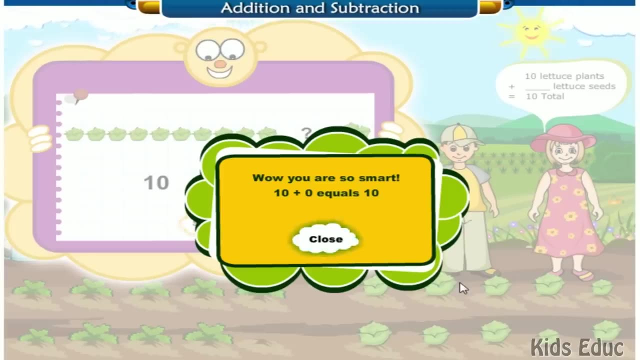 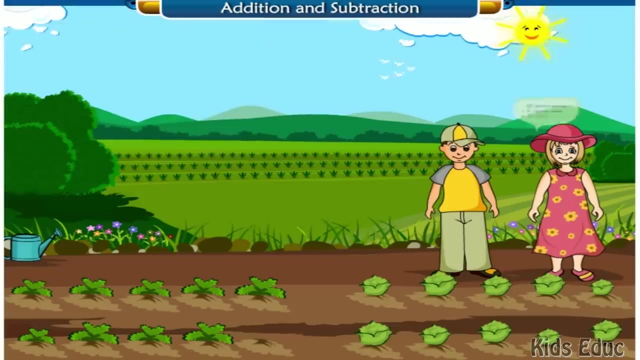 Let's do the math: 10 lettuce plants plus lettuce seeds equals 10 total. Wow, You are so smart. 10 plus 0 equals 10.. 10 lettuce plants plus 0 lettuce seeds equals 10 total. You are right. 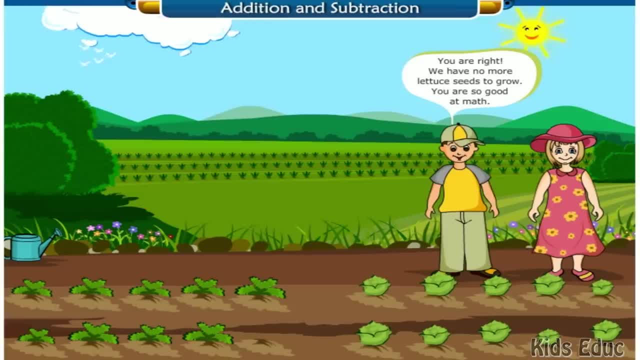 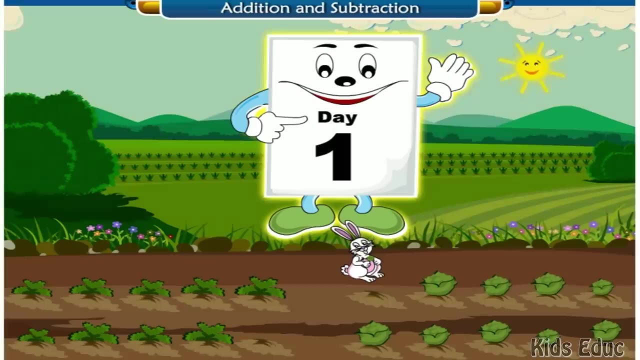 We have no more lettuce seeds to grow. You are so good at math. Let's water our garden, so all the seeds will grow big and strong. I want the water to be. I want the water to be inside of our garden, so all of the seeds can step out of the garden. 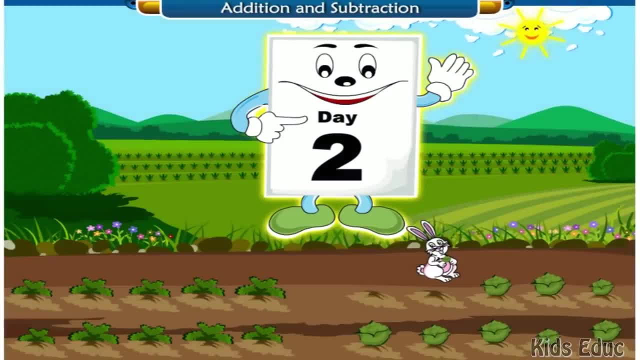 Look at me, física a limpo. My diseases have somewhat tastes terrible. How is that make a difference? I am still struggling to feel these consequences in my life. How am I in this world? What do we do? I will make something- meals for you instead of these 3. 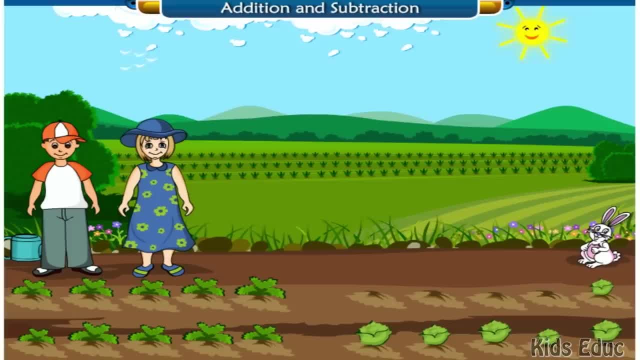 Hello Bunny Jose. how many carrot plants do we have? Let's count: One, two, three, four, five, six, seven, eight, nine, ten. We now have ten carrot plants. We planted ten carrot seeds and we now have ten carrot plants. 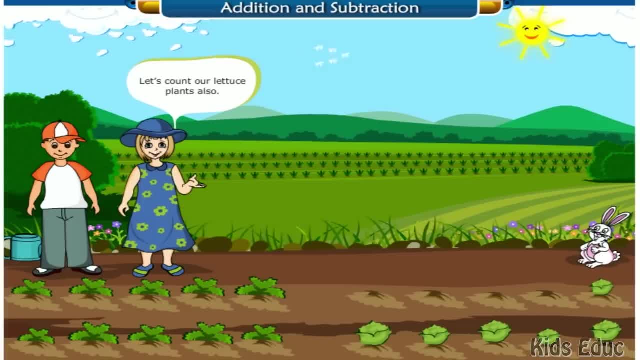 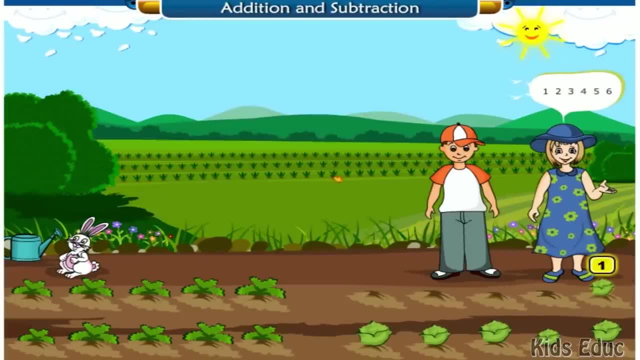 Yay, Let's count our lettuce plants also. One, two, three, four, five, six. We have six lettuce plants. Jose, how many lettuce plants did we have? When was the last time we visited the garden? We had all ten lettuce plants. 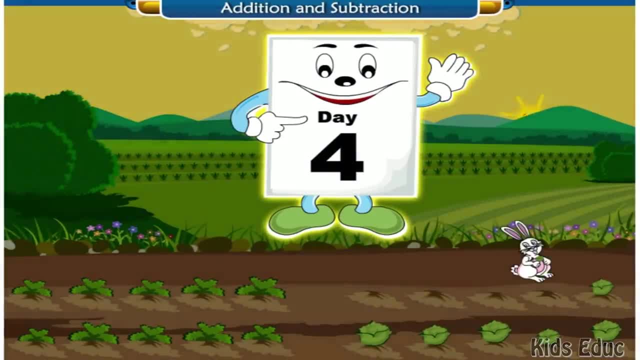 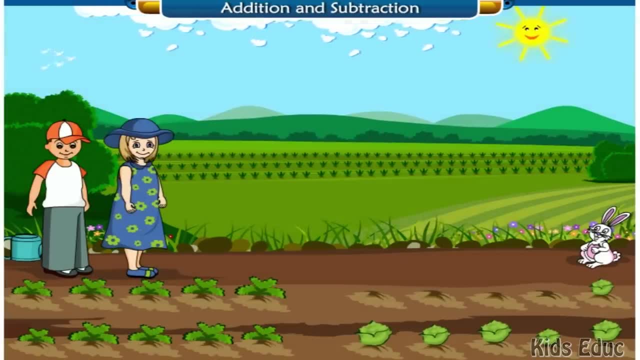 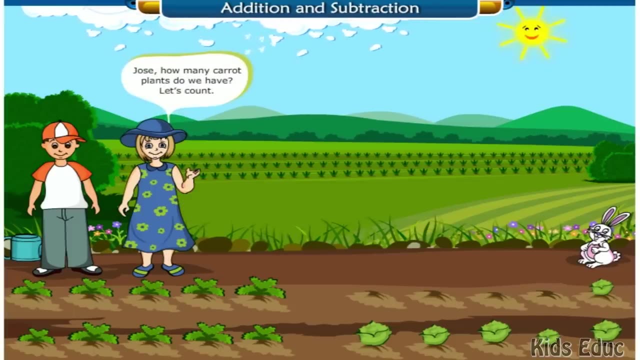 5. 6. 4. 5., 5., 6.. Wow, You are very smart. We now have to start aggi. opener Example. Let's do the math again and write down the number of 요아아ugs. 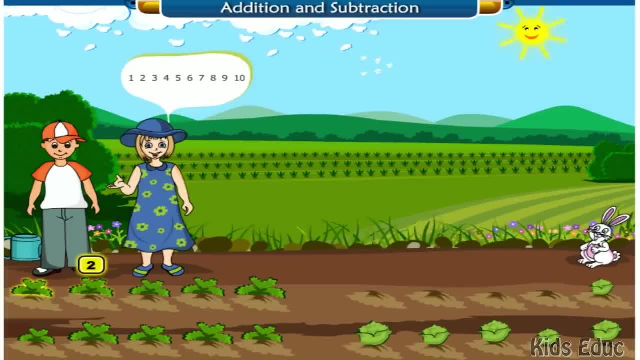 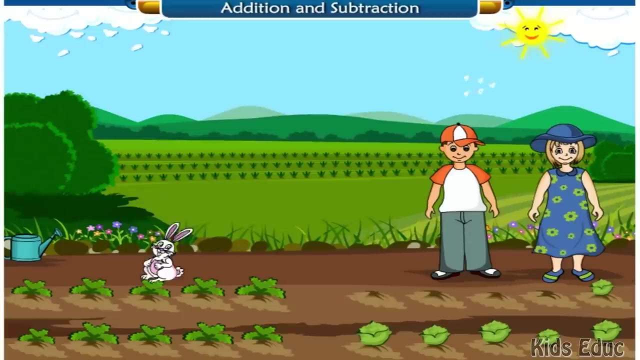 count one, two, three, four, five, six, seven, eight, nine, ten. we now have ten carrot plants. we planted ten carrot seeds and we now have ten carrot plants. yay, let's count our lettuce plants also: one, two, three, four, five, six. we have six lettuce plants. Jose, how many lettuce plants did we have the last time we visited the? 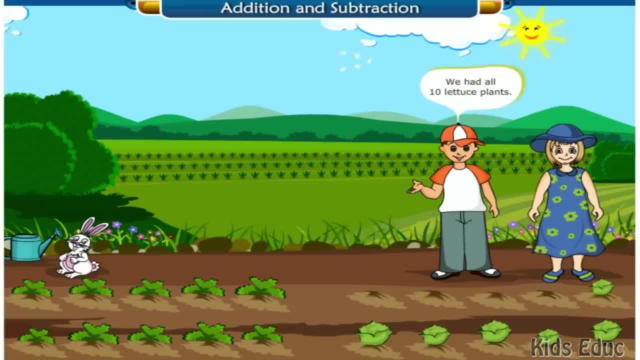 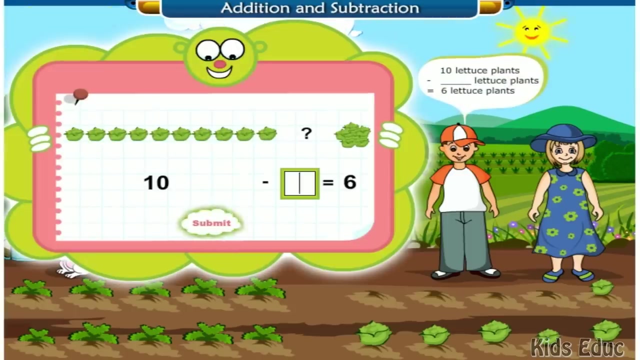 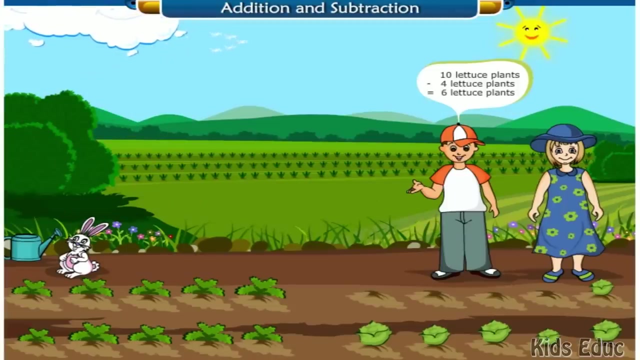 garden. we had all ten lettuce plants, Jose. how many are we missing? we started with ten lettuce plants and now we have six lettuce plants. let's do the math: ten lettuce plants minus lettuce plants equals six lettuce plants. ten minus four equals six. great job. ten lettuce plants minus four lettuce plants equals six lettuce plants. the. 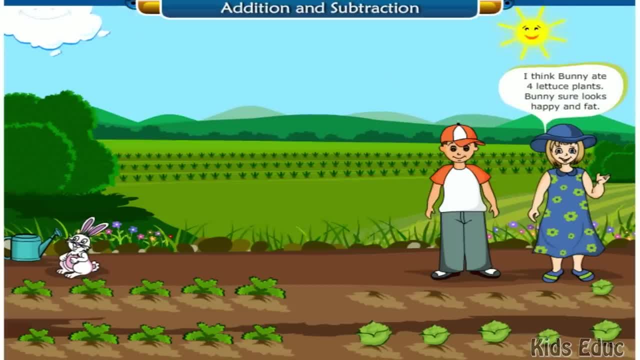 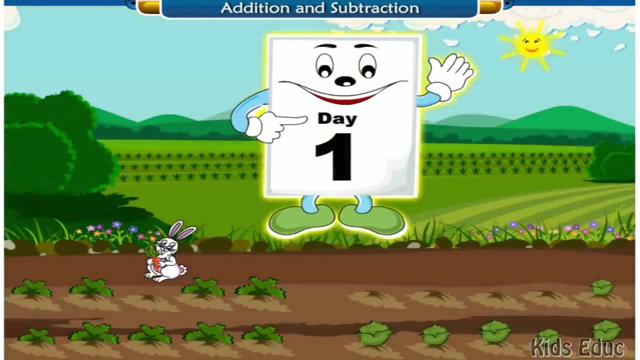 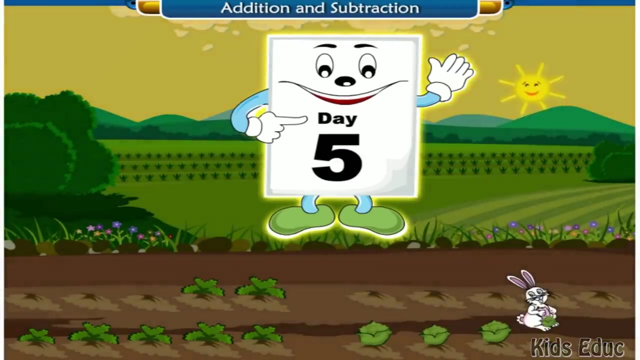 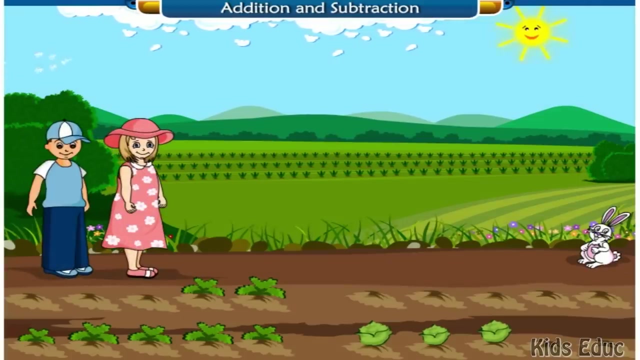 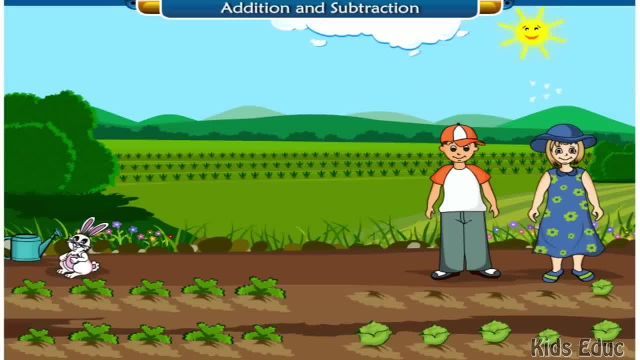 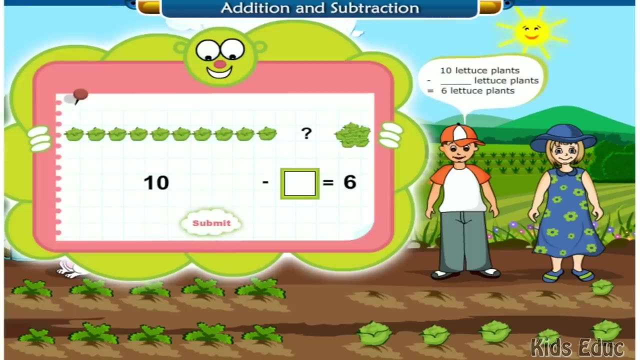 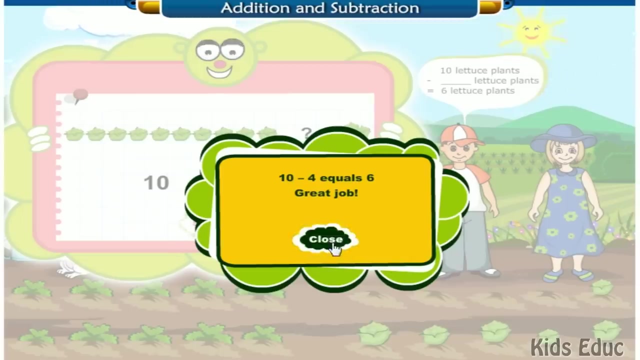 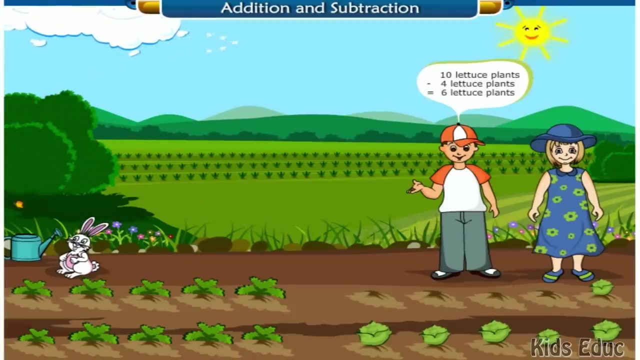 Jose, how many are we missing? We started with ten lettuce plants and now we have six lettuce plants. Let's do the math: Ten lettuce plants minus lettuce plants equals six lettuce plants. Ten minus four equals six. Great job. Ten lettuce plants minus four lettuce plants equals six lettuce plants. 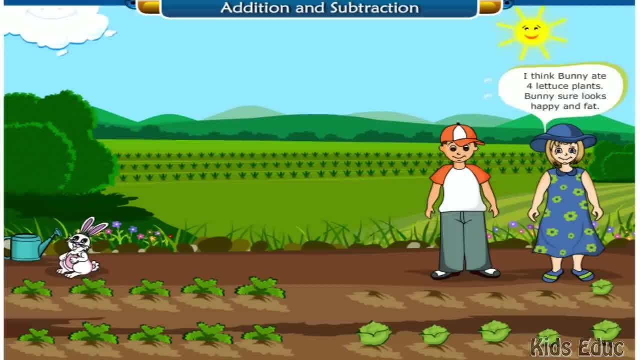 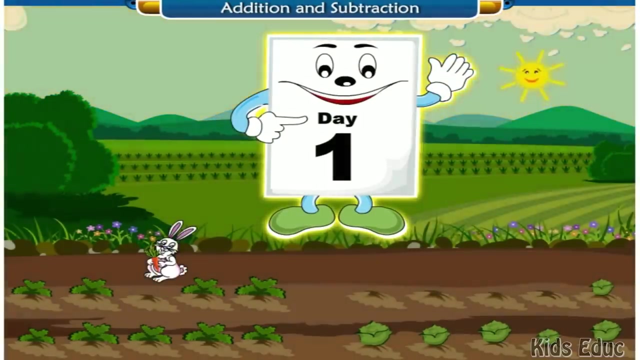 The answer is four. I think Bunny ate four lettuce plants. Bunny sure looks happy and fat. Oh well, We still have six lettuce plants growing. Let's water our garden so our plants can drink. Bunny neurologist. Bunny neurologist. Button neurologist. 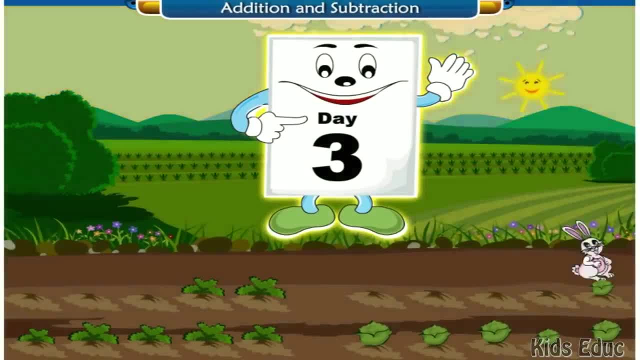 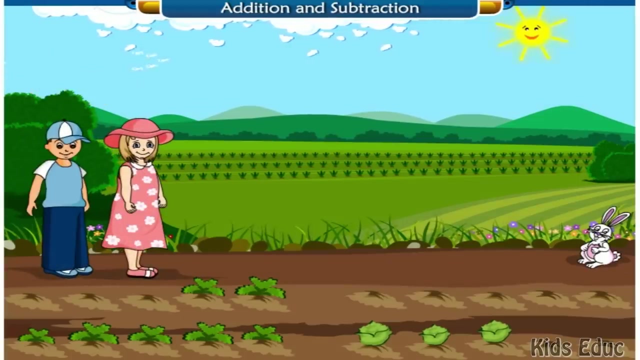 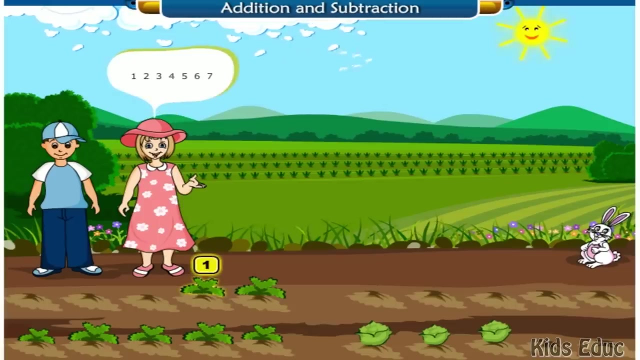 Point. armourологist- Internet neurologist. Hello, Bunny Jose. let's count our carrots today: 1,, 2,, 3,, 4,, 5,, 6, 7.. We now have 7 carrots. We had 10 carrots the last time we were in the garden. 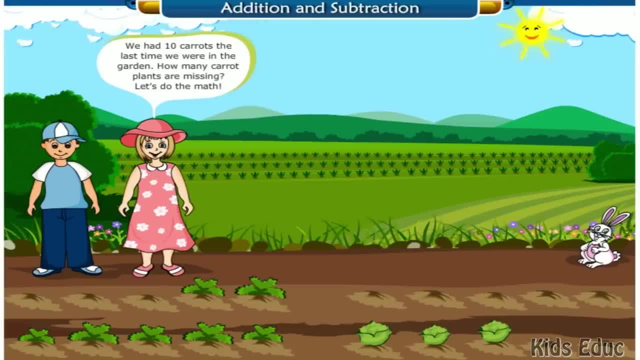 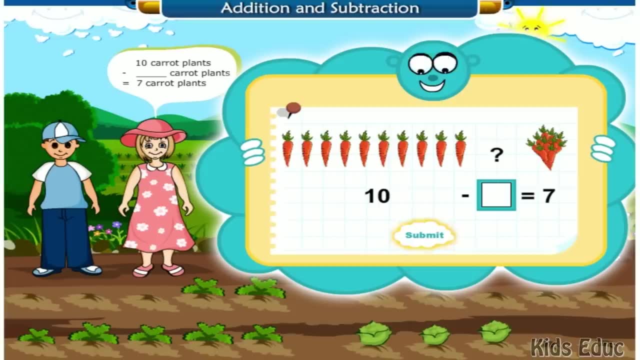 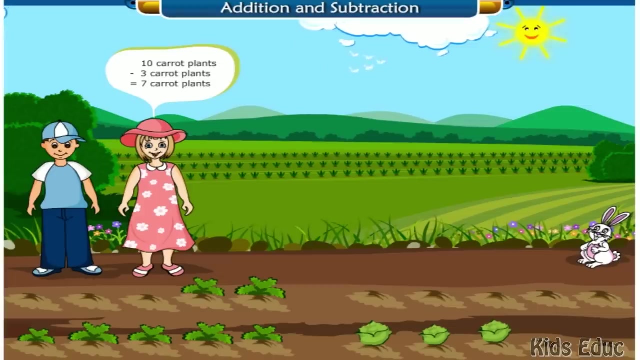 How many carrot plants are missing? Let's do the math: 10 carrot plants minus carrot plants equals 7.. 7 carrot plants: 10 minus 3 equals 7.. Great math: 10 carrot plants minus 3 carrot plants equals. 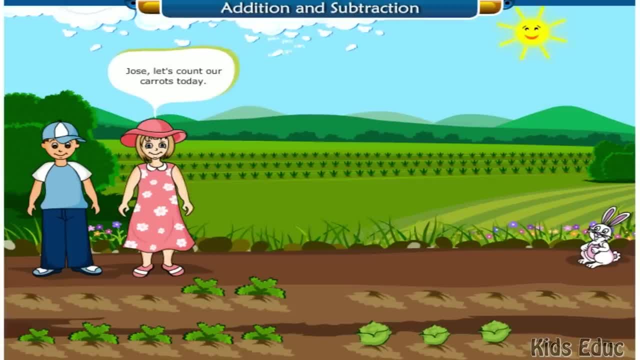 Jose, let's count our carrots today: One, two, three, four, five, six, seven. We now have seven carrots. We had ten carrots the last time we were in the garden. How many carrot plants are missing? Let's do the math. 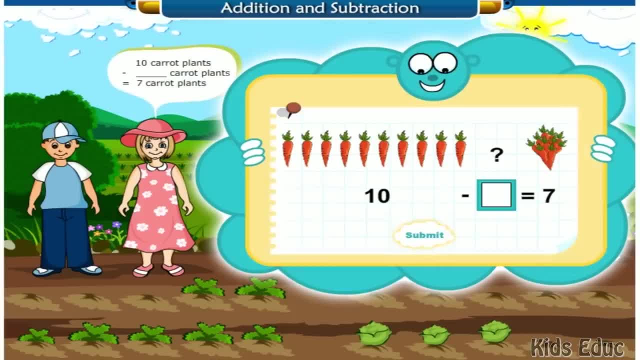 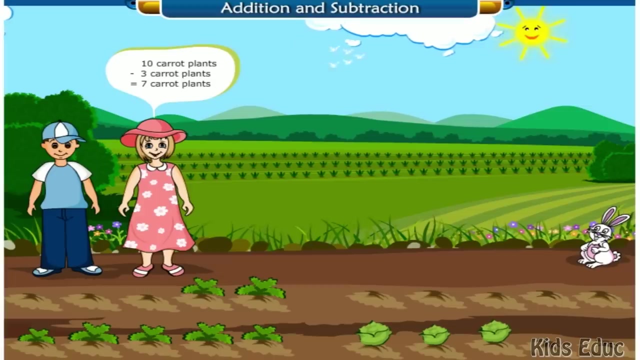 Ten carrot plants minus carrot plants equals seven carrot plants. Ten minus three equals seven. Great math: Ten carrot plants minus three carrot plants equals seven carrot plants. The answer is three. I bet Bunny ate the three missing carrots. Bunny sure looks happy. 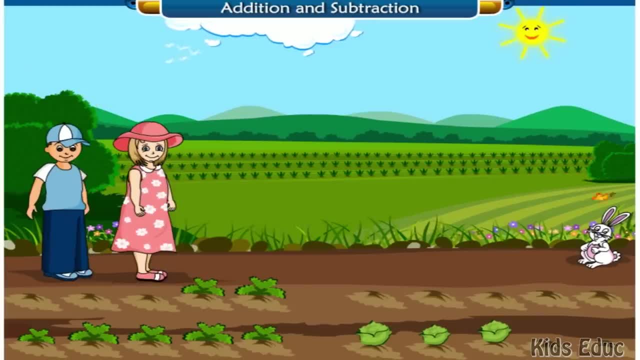 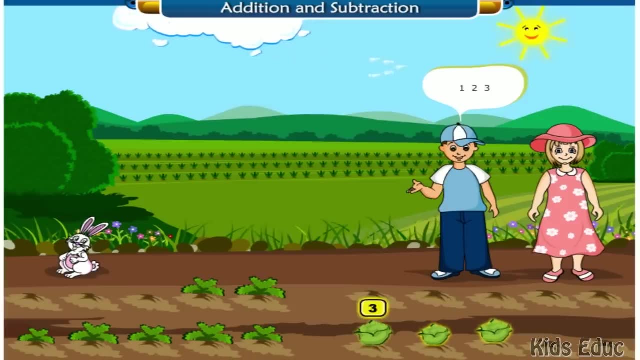 Let's count our lettuce plants. Let's count our lettuce plants: One, two, three, four, five, six, seven. One, two, three. We only have three lettuce plants left. How many lettuce plants did we have the last time we checked our garden? 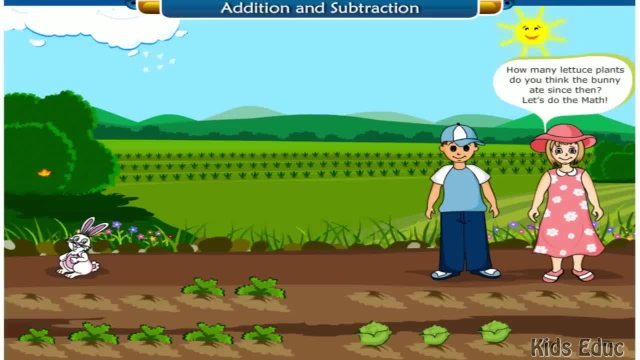 We had six lettuce plants. How many lettuce plants do you think the bunny ate since then? Let's do the math. We started out with six lettuce plants and now we have only six. We have only three lettuce plants left. Hmm, Let's do the math. 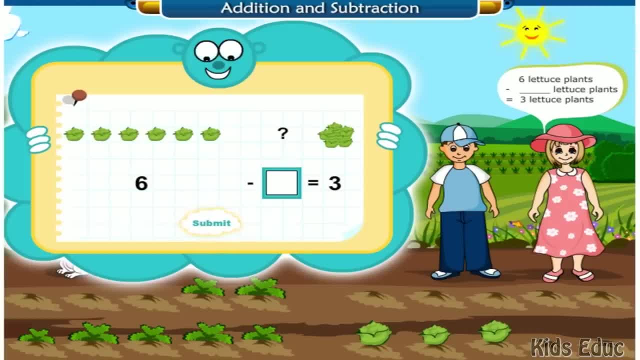 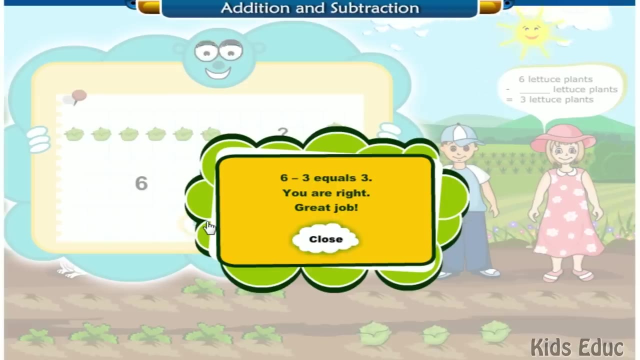 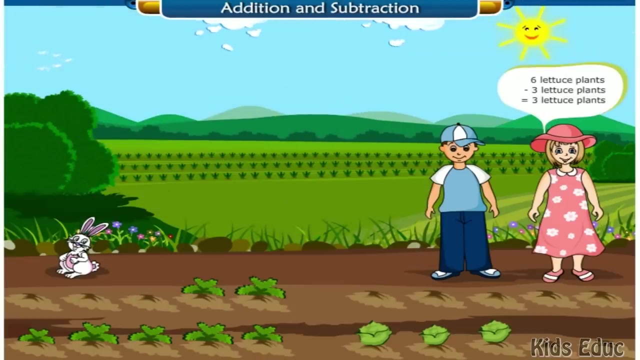 Six lettuce plants minus lettuce plants equals three lettuce plants. Six minus three equals three. You are right, Great job. Six lettuce plants minus three lettuce plants equals three lettuce plants. You are right, Great job. The answer is three, You are right. 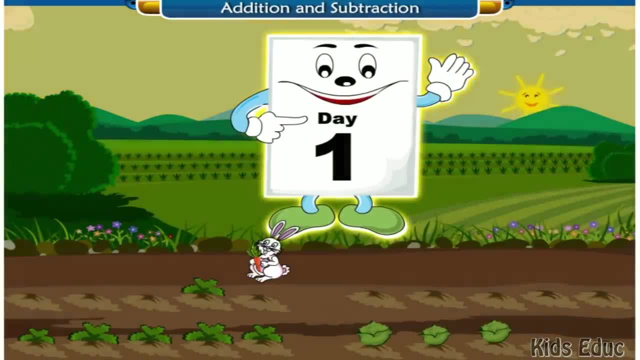 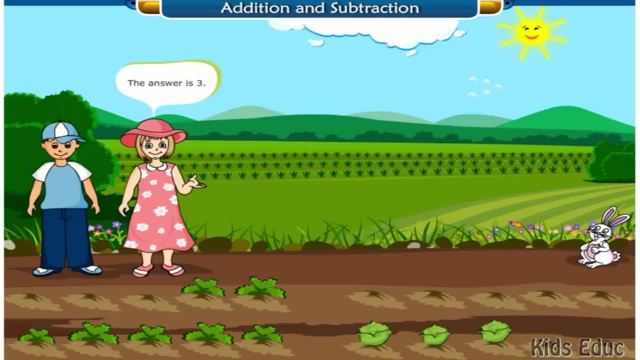 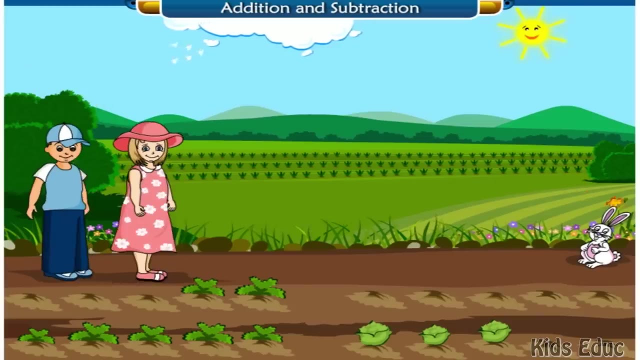 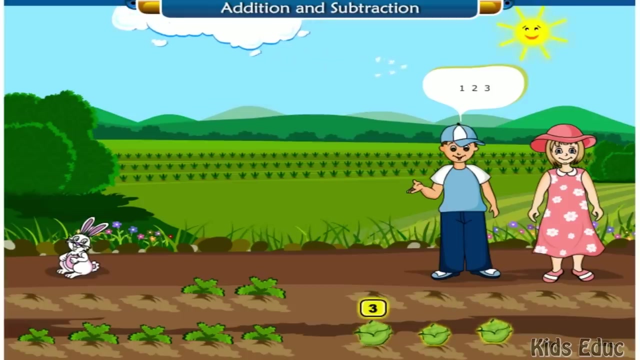 7 carrot plants, The answer is 3.. I bet Bunny ate the 3 missing carrots- Carrots. Bunny sure looks happy. Let's count our lettuce plants: 1,, 2,, 3.. We only have 3 lettuce plants left. 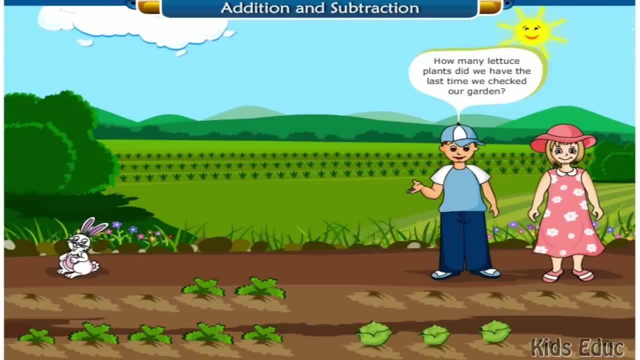 How many lettuce plants did we have? the last time we checked our garden, We had 6 lettuce plants. How many lettuce plants do you think the bunny ate since then? Let's do the math: We started out with 6 lettuce plants and now we have only 3 lettuce plants left. 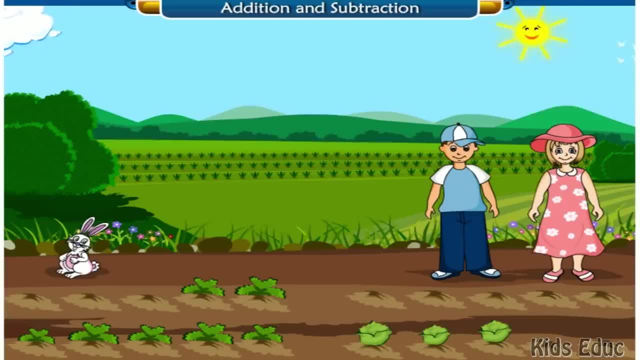 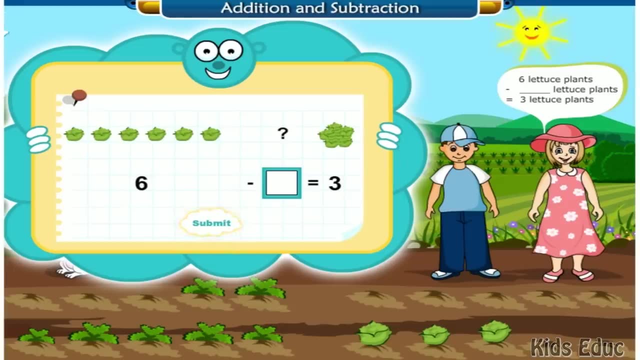 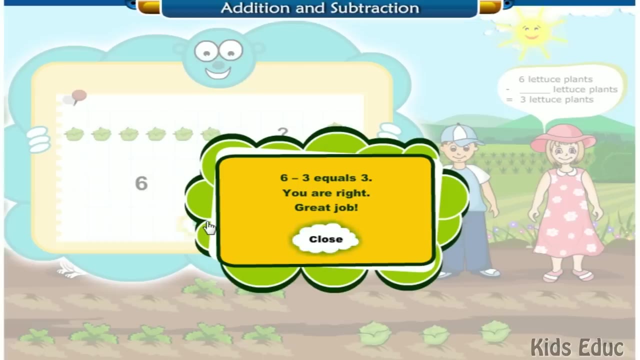 Hmm, Let's do the math: 6 lettuce plants minus lettuce plants equals 3 lettuce plants. 6 means lie, 6 minus 3.. 5 minus 3 equals 3.. We're само-be, just like Dr Viking. 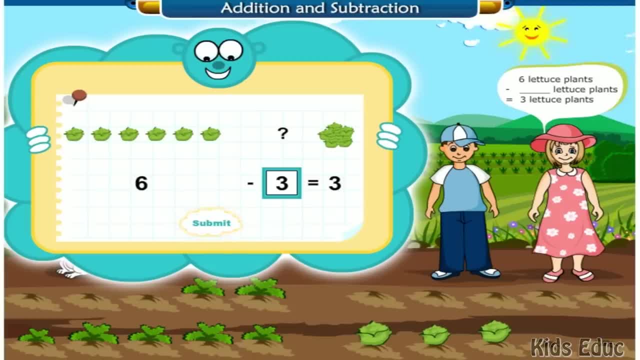 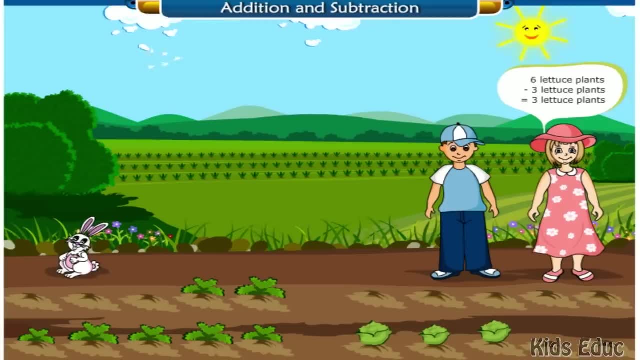 You are right, Great job. Math question. Go easy with your math questions. 6 lettuce plants minus 3 lettuce plants equals 3 lettuce plants. You are right, Great job. The answer is 3.. Remember that, No Ifs and Buts. 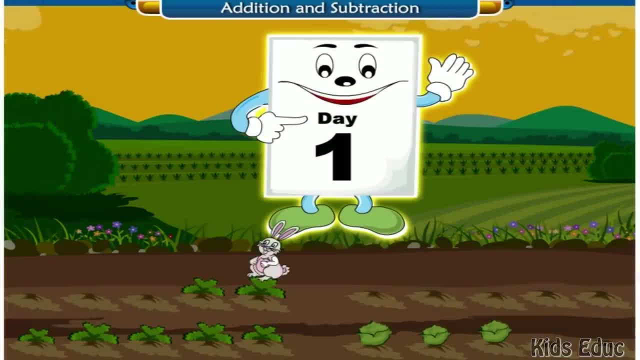 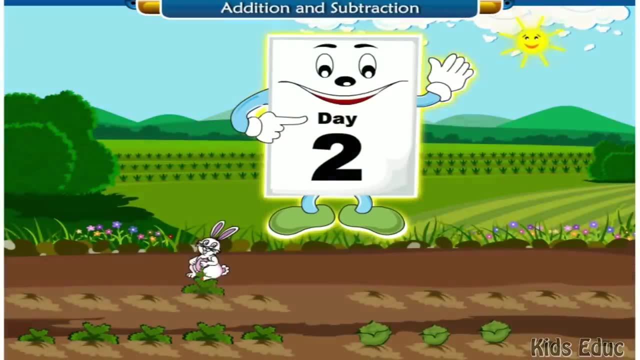 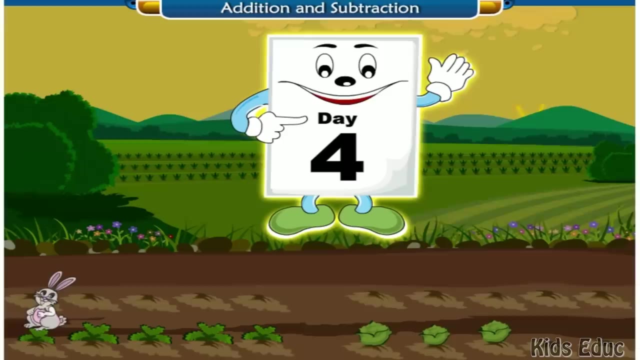 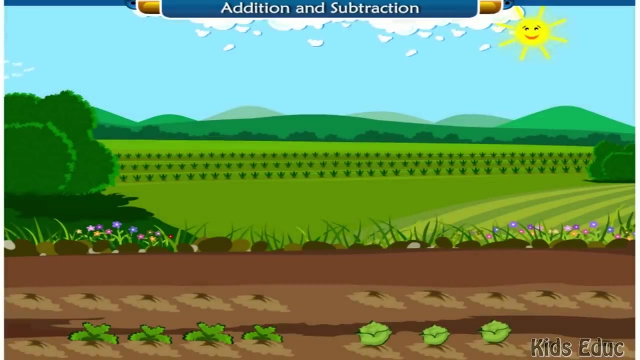 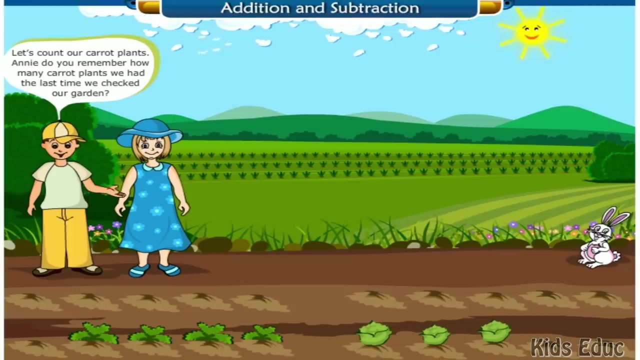 Let's count our carrot plants. Annie, do you remember how many carrot plants we had the last time we checked our garden? Yes, we had seven carrot plants left. Well, let's count our carrots today: One, two, three, four. 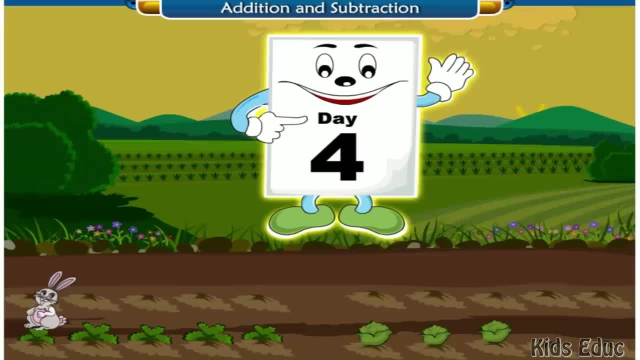 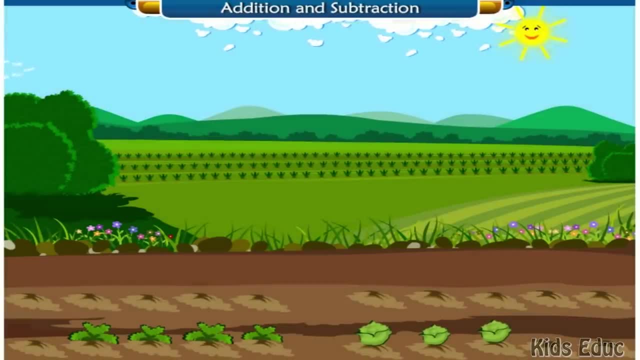 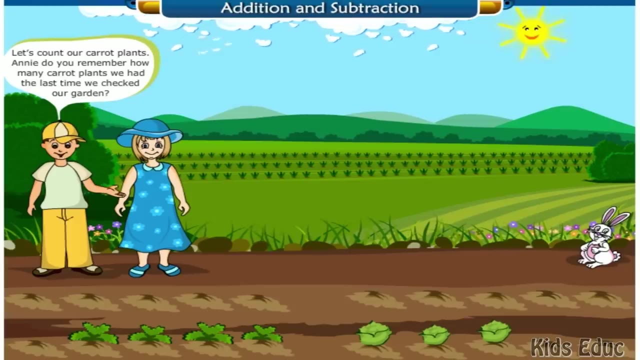 The answer is three. You are right. Great job. Let's count our carrot plants. Annie, do you remember how many carrot plants we had the last time we checked our garden? Yes, we had seven carrot plants left. Well, let's count our carrots today. 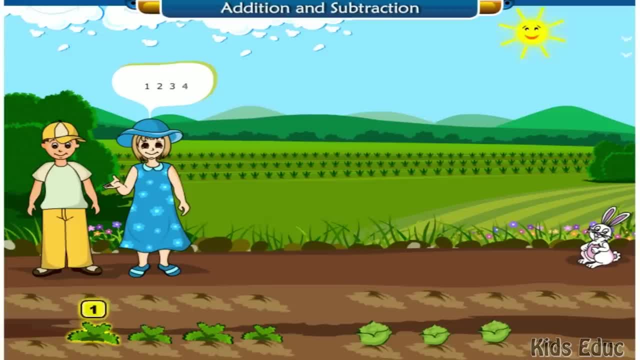 One, two, three, four. We only have four carrot plants left. Oh, my goodness, I think we have a very hungry bunny. How many more carrots did he eat? Let's do the math If we started out with seven carrots and now we have only four left? 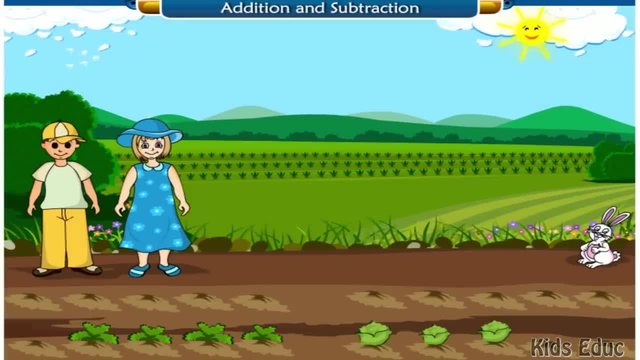 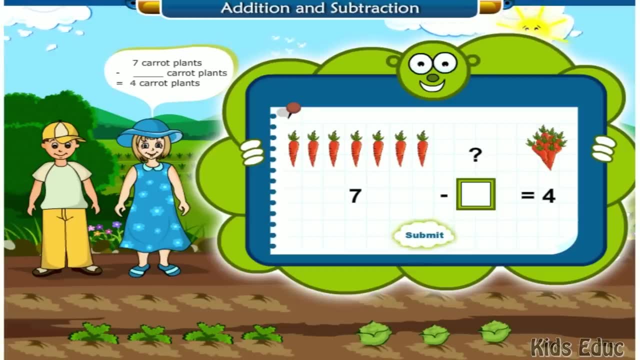 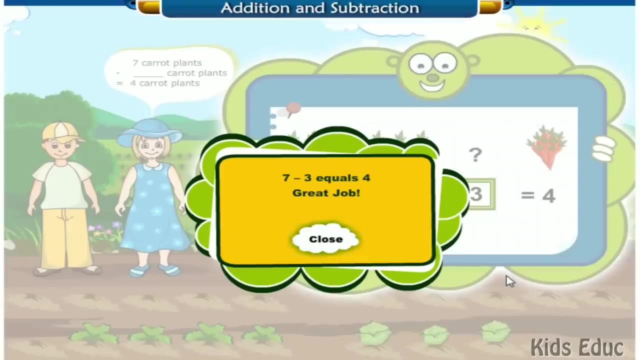 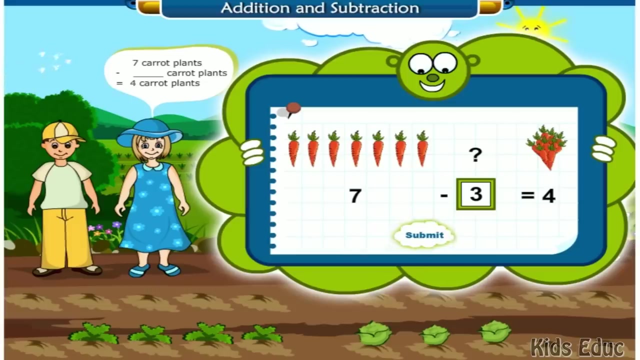 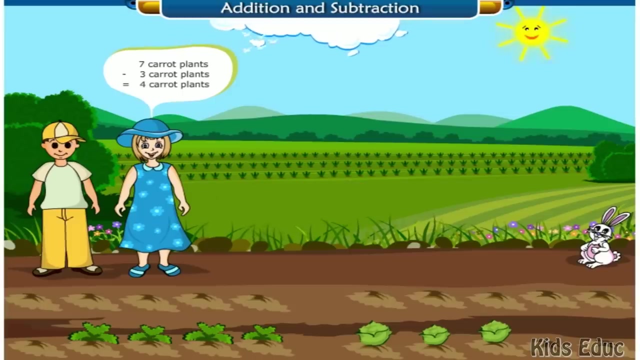 how many carrots did he eat? How many carrots are missing? Seven carrot plants minus carrot plants equals four carrot plants. Seven minus three equals four. Great job. Seven carrot plants minus three carrot plants Equals four carrot plants. The answer is three. 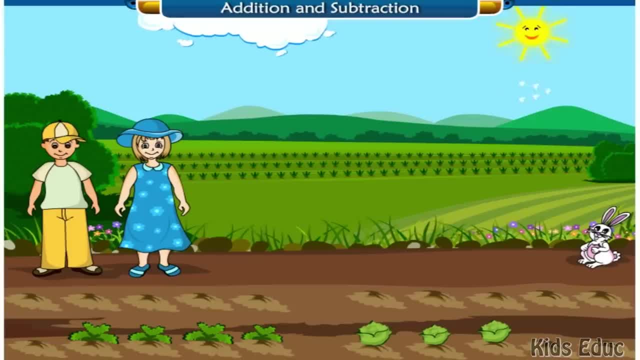 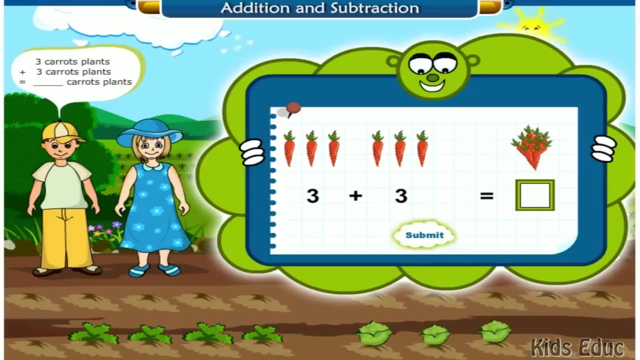 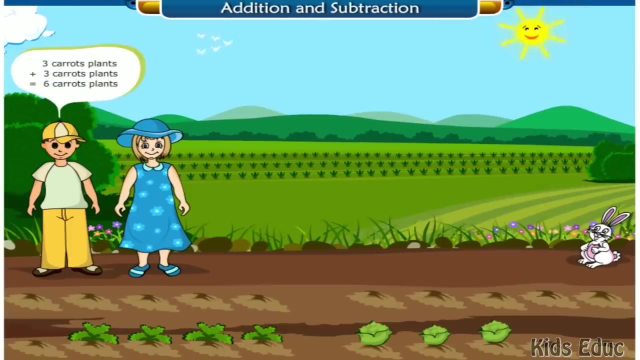 How many carrots has bunny eaten? Well, he first ate three carrots and now he has eaten three more. So let's do the math. Three carrot plants plus three carrot plants equals carrot plants. Three plus three equals six. Great job. Three carrot plants plus three carrot plants equals six carrot plants. 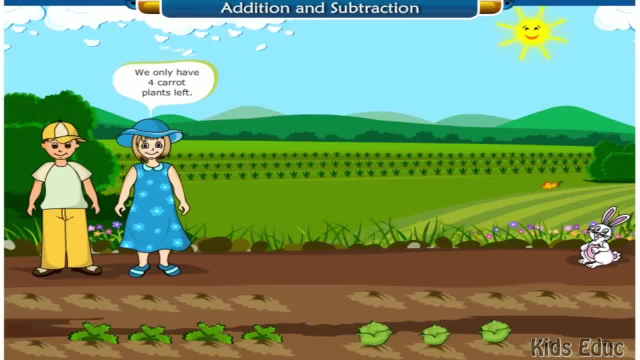 We only have four carrot plants left. Oh, my goodness, I think we have a very hungry bunny. How many more carrots did he eat? Let's do the math: If we started out with seven carrots and now we have only four left, how many carrots are missing? 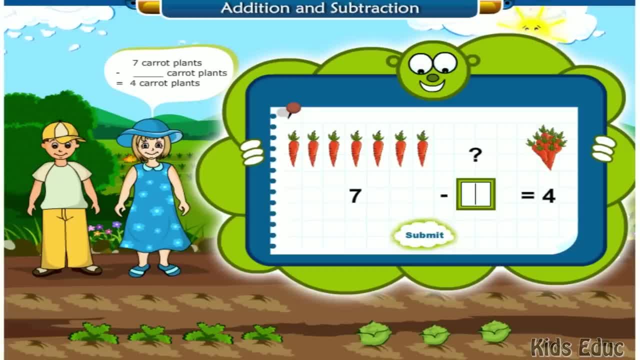 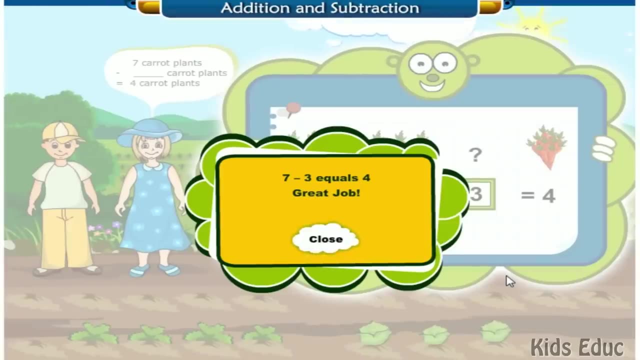 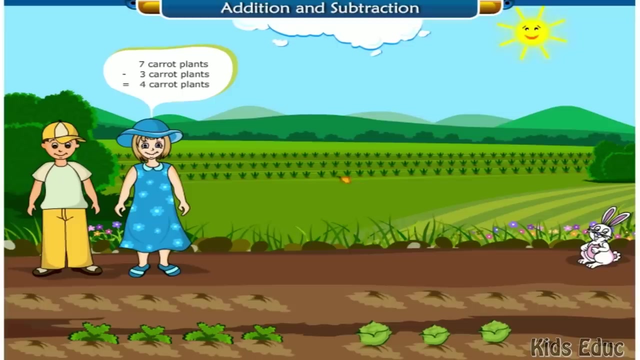 Seven carrot plants minus carrot plants equals four carrot plants. Seven minus three equals four. Great job. Seven carrot plants minus three carrot plants equals four carrot plants. The answer is three. How many carrots has bunny eaten? Well, he first ate three carrots. 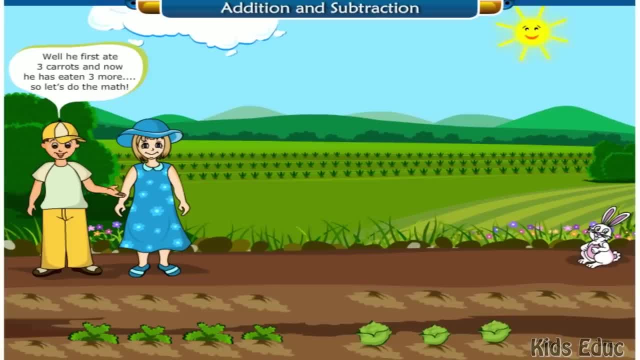 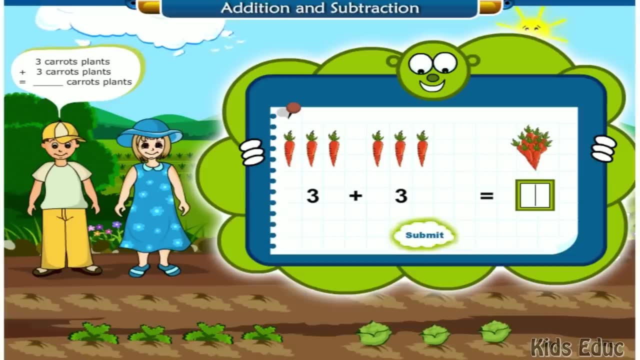 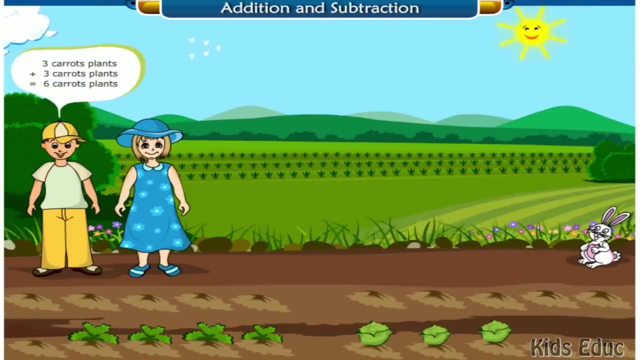 and now he has eaten three more. So let's do the math: Three carrot plants plus three carrot plants equals carrot plants. Three plus three equals six. Great job, Great job. Three carrot plants plus three carrot plants equals six carrot plants. Six is the correct answer. 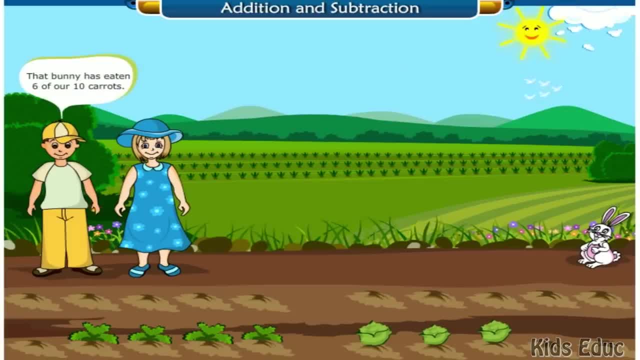 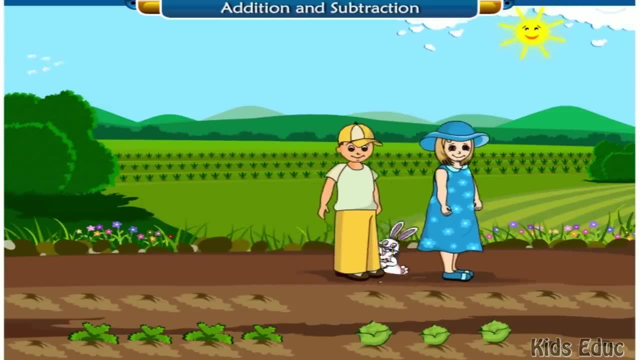 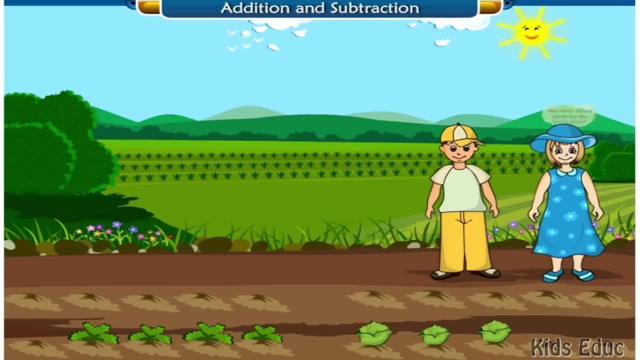 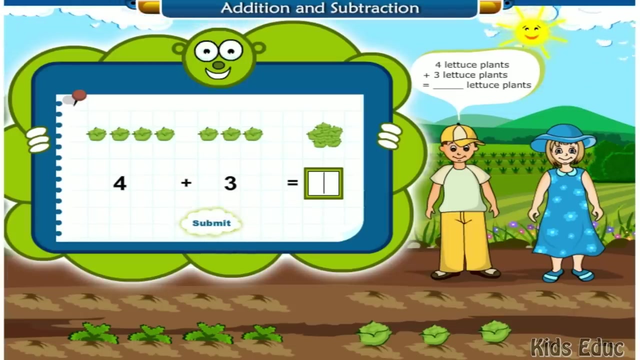 That bunny has eaten six of our ten carrots. He must be a very hungry bunny. How many lettuce plants has the bunny eaten? Well, he first ate four and then he ate three more lettuce plants. So let's do the math: Four lettuce plants plus three lettuce plants equals lettuce plants. 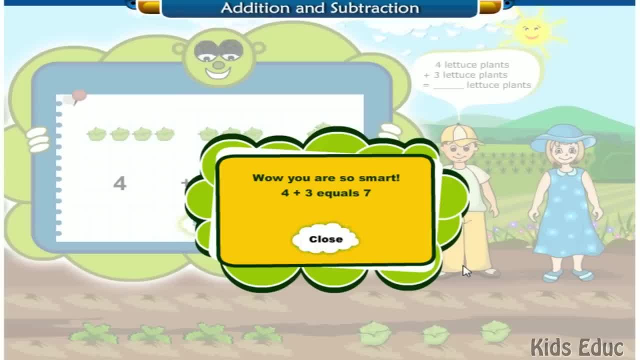 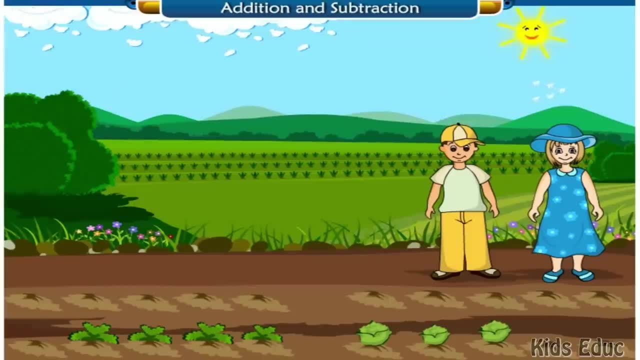 Wow, you are so smart. Four plus three equals six. Three plus three equals seven. Four lettuce plants plus three lettuce plants equals seven lettuce plants. Bunny has eaten seven lettuce plants and six carrots. Wow, bunny sure is hungry. How can one bunny be so hungry?